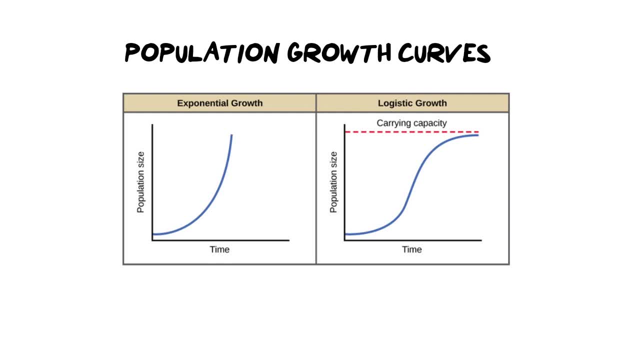 get full marks in your finals and any of your tests and exams that you write. I also have a grade 12 study guide that you can use to get a copy of my grade 11 study guide. I also have a 12 one- if you're looking into the future as well- which is filled with all of my top tips for finals. 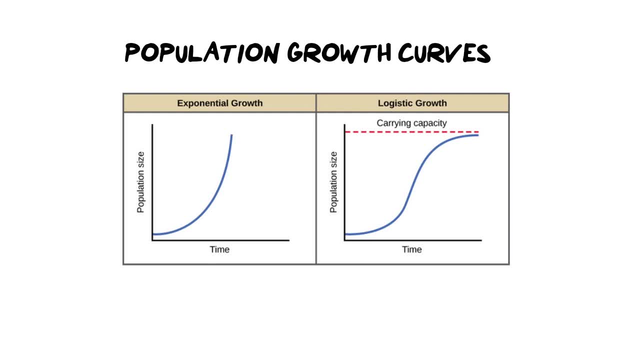 as well, and you can get a copy of that on my website, which is missanglacoza. Now, today, what we're going to cover is these two major growth curves that you can see in front of you. We're going to look at exponential growth. I'm going to look at a logistic growth. There is a lot of 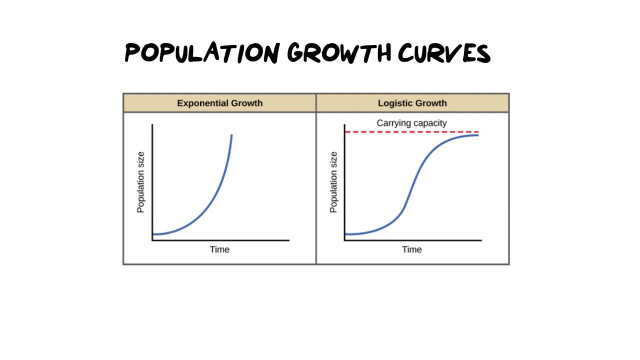 things that are playing sort of in the background of these growth curves, and what that means is you need a lot of knowledge about habitats, competition and how, basically, survival of the fidgets works in order for these two graphs to be drawn. Now, before we get into the deeper explanations, what? 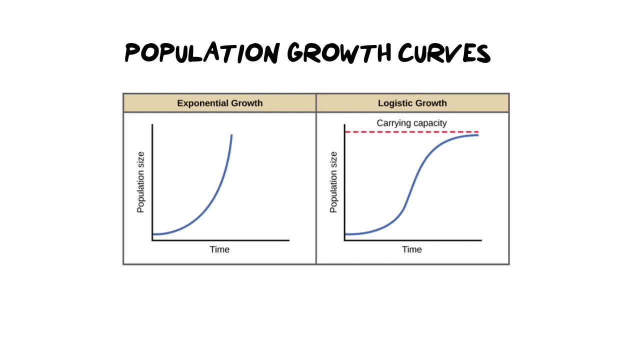 I want to cover is two major words that you see very, very often. One of them is going to be this guy over here carrying capacity, like what actually is it, and because it's really important for populations. and two, how do you make that carrying capacity and what is it? how was it formed? we're 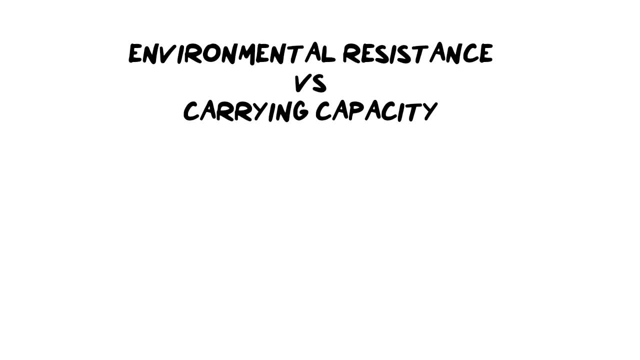 going to look at that now too. So, as I mentioned earlier, it's a really, really, really big deal to know the difference between your terminology in this section, and two of the words that are often confused with each other are environmental resistance and carrying capacity. They are 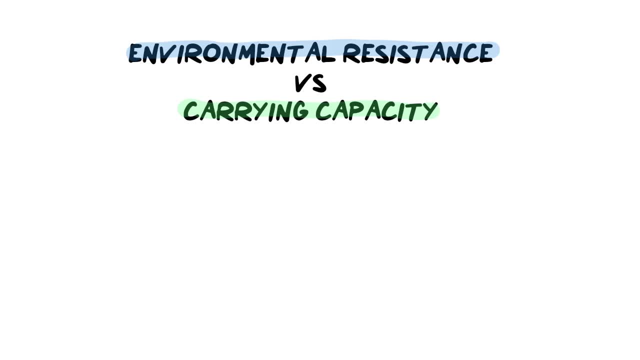 definitely not the same thing, and too many people confuse them with one another, and I'm going to show you the differences between the two and then I'm going to show you how they interact with one another. So let's start off with the environmental resistance aspect of our population Now, every single population when it's growing. in the beginning. 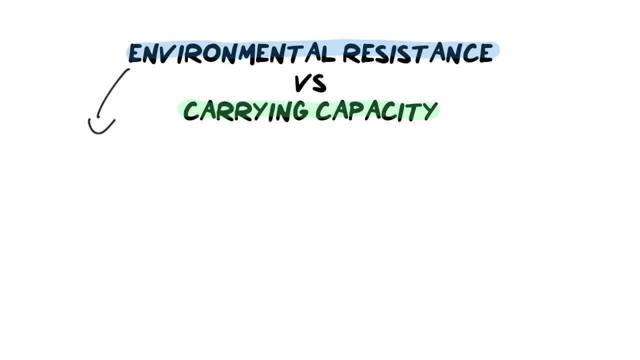 it doesn't have to worry about resources because the population is small, so they flourish. However, over time, the environment is going to resist the growth of the population because the resources become limited over time, and these resources can be things like water, food, sunlight, space, shelter, mates, etc. And so the environment resists the growth. 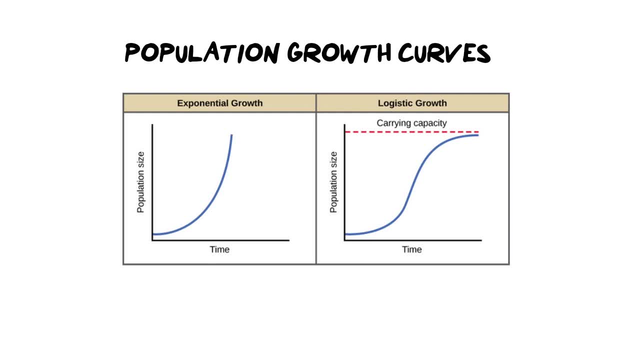 as well, and you can get a copy of that on my website, which is missanglacoza. Now, today, what we're going to cover is these two major growth curves that you can see in front of you. We're going to look at exponential growth. I'm going to look at a logistic growth. There is a lot of 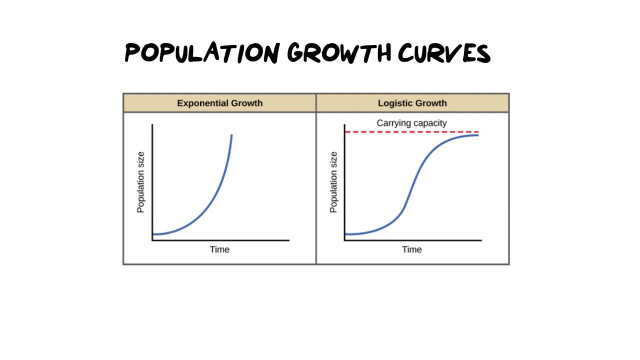 things that are playing sort of in the background of these growth curves, and what that means is you need a lot of knowledge about habitats, competition and how, basically, survival of the fidgets works in order for these two graphs to be drawn. Now, before we get into the deeper explanations, what? 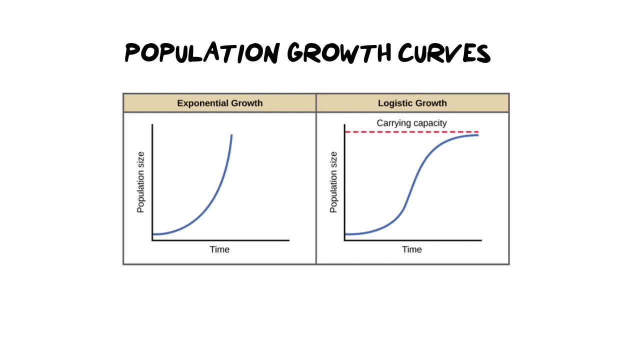 I want to cover is two major words that you see very, very often. One of them is going to be this guy over here carrying capacity, like what actually is it, and because it's really important for populations. and two, how do you make that carrying capacity and what is it? how was it formed? we're 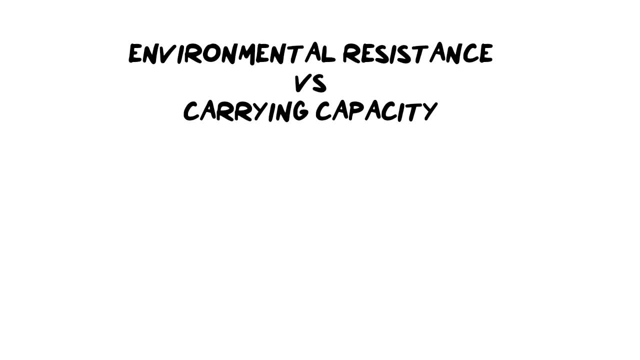 going to look at that now too. So, as I mentioned earlier, it's a really, really, really big deal to know the difference between your terminology in this section, and two of the words that are often confused with each other are environmental resistance and carrying capacity. They are 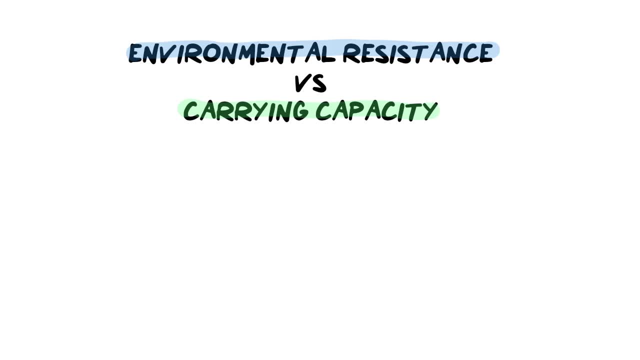 definitely not the same thing, and too many people confuse them with one another, and I'm going to show you the differences between the two and then I'm going to show you how they interact with one another. So let's start off with the environmental resistance aspect of our population Now, every single population when it's growing. in the beginning. 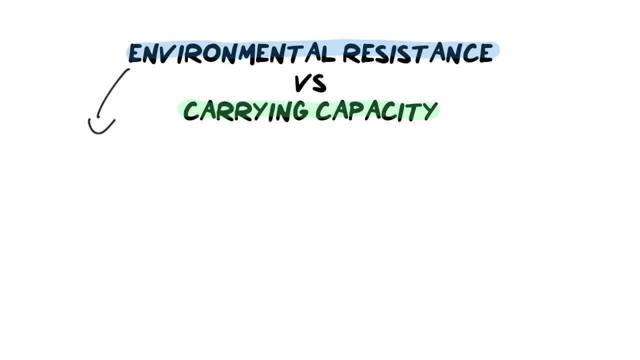 it doesn't have to worry about resources because the population is small, so they flourish. However, over time, the environment is going to resist the growth of the population because the resources become limited over time, and these resources can be things like water, food, sunlight, space, shelter, mates, etc. And so the environment resists the growth. 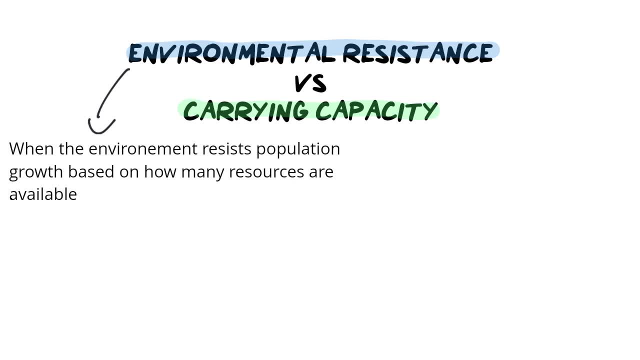 of the population. Now, when it resists the population, it creates a level or a maximum amount of individuals that the ecosystem can support, which is what we call the carrying capacity. So, in other words, the carrying capacity is met when there is a balance between the biotic or the living population and its 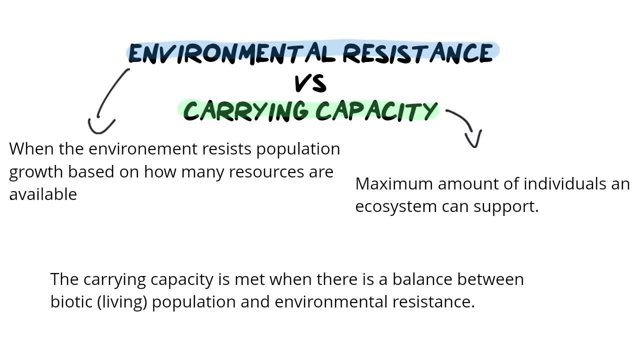 environmental resistance. So the resistance is what makes the carrying capacity. It's almost, if you think of it like this, the environmental resistance is the process and the carrying capacity is the growth of the population. So the environmental resistance is the process and the product. It's the thing that we create. I want you to know also that when we look at a graph, often the 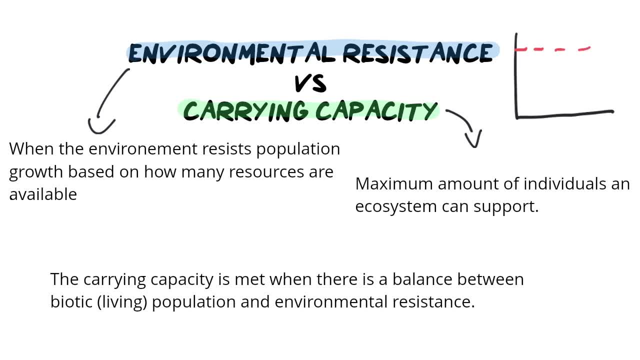 carrying capacity is included as the sort of like dotted line, and you will notice that the population often goes above it and then sort of fluctuates around it and they even level off. I want you to know that the carrying capacity can actually move down and it can also move up, and it can also move up. 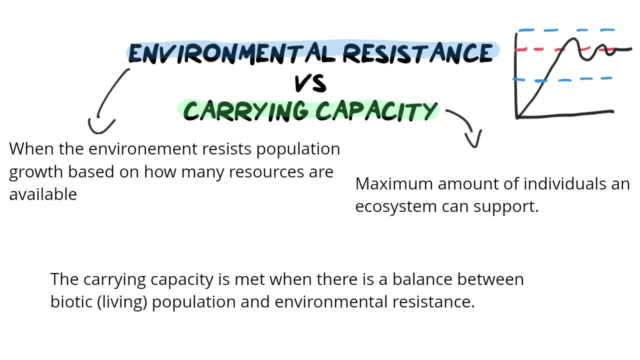 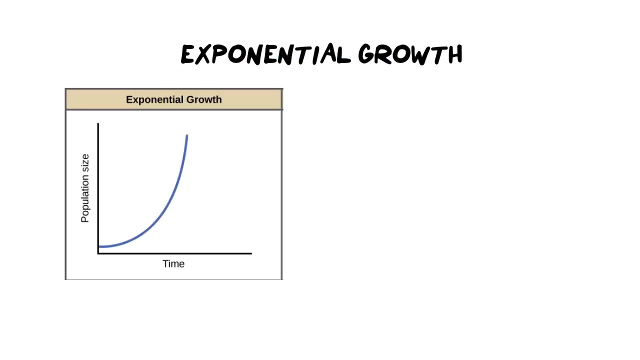 Depending on the environmental resistance, which means if there are fewer resources, the carrying capacity moves down. If there are more resources, the carrying capacity will move up, and so it all is a fine balance between the living components, which is the population, and then of course, the non-living things, like their space, shelter, water, etc. So let's have a look at the first type of 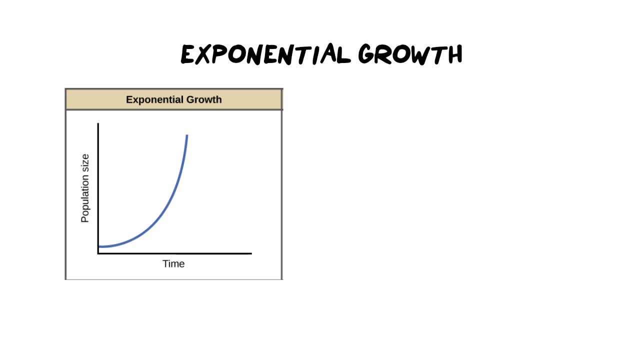 growth that we see in populations And it is called exponential growth and it is characterized by this sort of J shape that it produces when you plot the points. Of course we are plotting over time and population size. Now there are some key things that we need to keep in mind when we look at exponential growth. 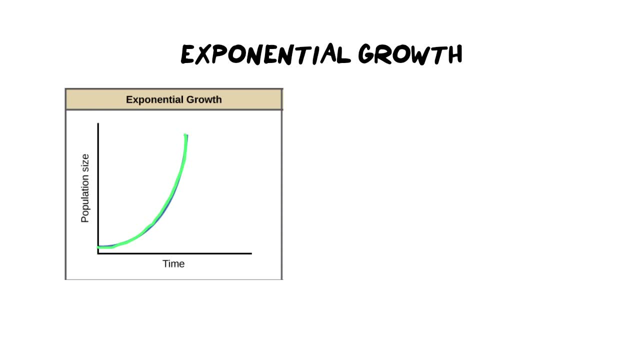 and I want you to look out for these things when you have to explain what is happening. So exponential growth often occurs in a population that is not a population, That is starting off quite small. Maybe they are new to the environment or maybe the environment 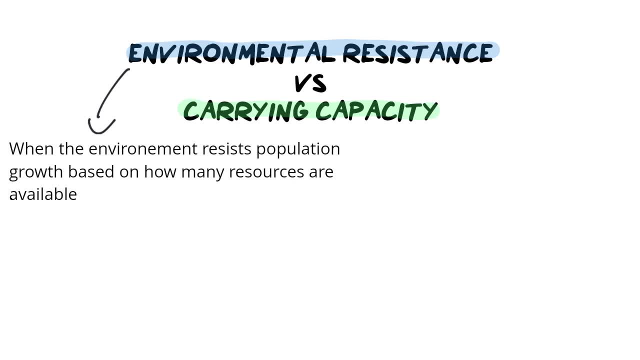 of the population. Now, when it resists the population, it creates a level or a maximum amount of individuals that the ecosystem can support, which is what we call the carrying capacity. So, in other words, the carrying capacity is met when there is a balance between the biotic or the living population and its 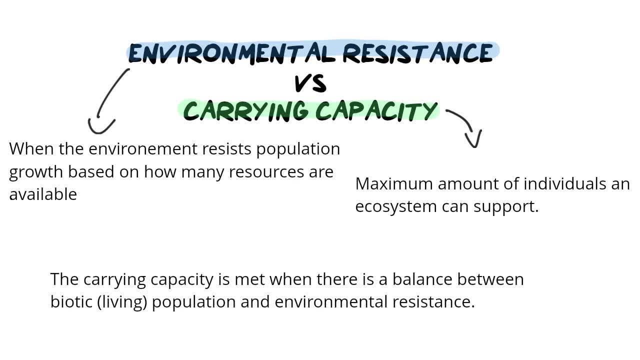 environmental resistance. So the resistance is what makes the carrying capacity. It's almost, if you think of it like this, the environmental resistance is the process and the carrying capacity is the growth of the population. So the environmental resistance is the process and the product. It's the thing that we create. I want you to know also that when we look at a graph, often the 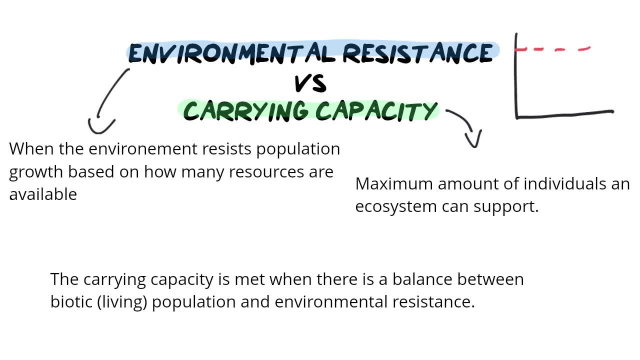 carrying capacity is included as the dotted line and you will notice that the population often goes above it and then fluctuates around it and may even level off. I want you to know that the carrying capacity can actually move down and it can also move up, depending on the environmental resistance, which means if there are fewer resources, the carrying 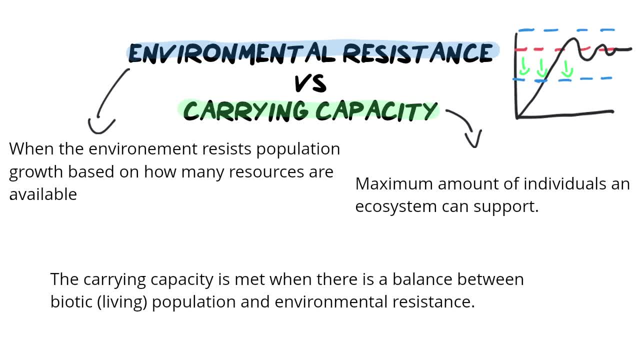 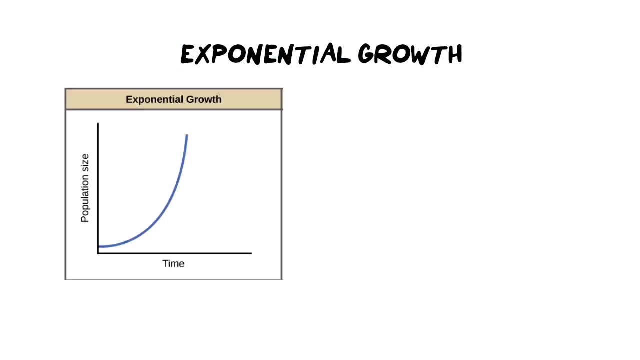 capacity moves down. If there are more resources, the carrying capacity will move up, and so it all is a fine balance between the living components, which is the population, and then, of course, the non-living things, like their space, shelter, water, etc. So let's have a look at the first type of 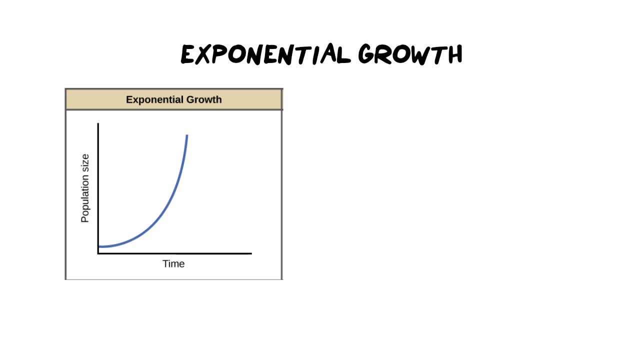 growth that we see in populations And it is called exponential growth and it is characterized by this sort of J shape that it produces when you plot the points. Of course we are plotting over time and population size. Now there are some key things that we need to keep in mind when we look at exponential growth. 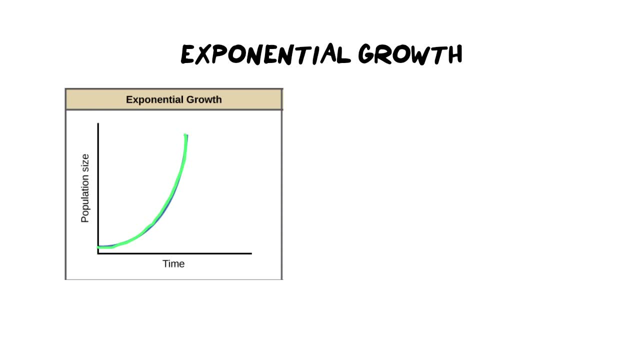 and I want you to look out for these things when you have to explain what is happening. So exponential growth often occurs in a population that is not a population, That is starting off quite small. Maybe they are new to the environment or maybe the environment 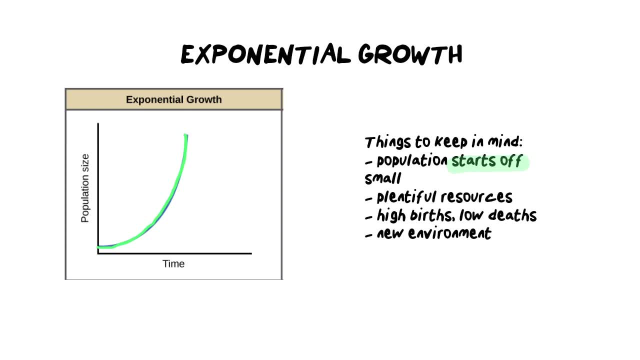 itself is new, and so they are starting off with maybe four or five breeding pairs. There's not going to be a lot of individuals. What's also important in the exponential growth curve is: you must acknowledge that there is plentiful resources. The reason that we know that is because, if we look 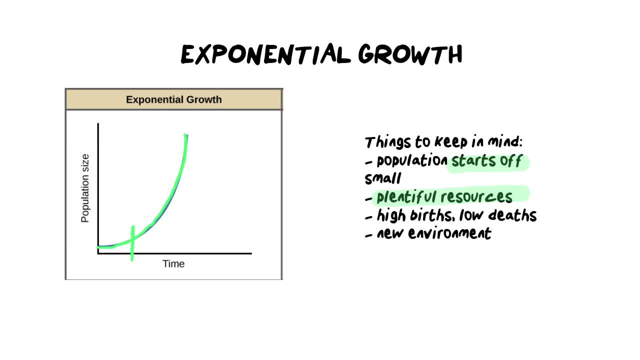 at the graph in the beginning, this First sector. over here the growth is quite slow and gradual and that is because the amount of breeding pairs are limited and reproduction takes time, and you know, just in general populations take a little while to establish. However, everything after that is exponential, Like there's a sharp 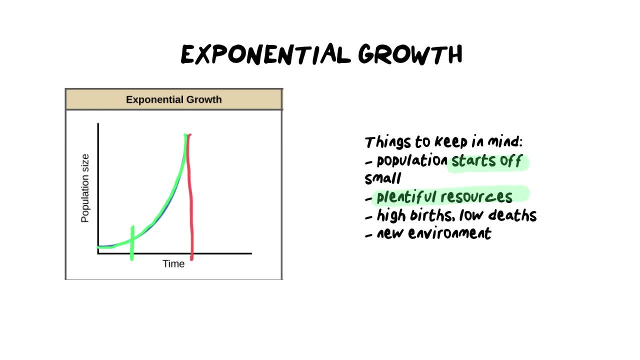 increase over a very short period of time. That is because there are so many resources available, Very little disease, Very little competition. Everybody has enough of everything to reproduce at their maximum, and so that's why we see a high birth, low death rate. Now, the last thing I want you to keep in mind is exponential growth. 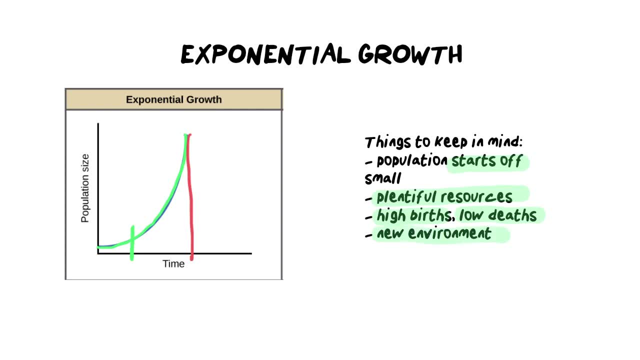 happens often in a new environment. It basically means maybe this organism didn't live there before, and now they're newly introduced, or an area that used to have them has been cleared out, More space has been provided to them and now they have, you know, like an area to establish. 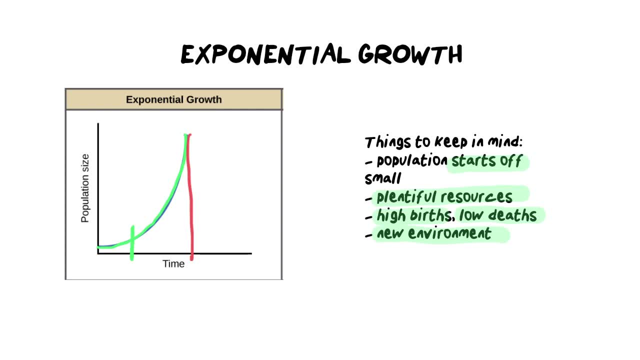 themselves, And often we see exponential growth in organisms like bacteria. We see these in like rodents and mice or butterflies. There's like an explosion of growth. And then what is missing in this graph, which I'm going to include for us now, is what we call a drop off point, And I'm going to 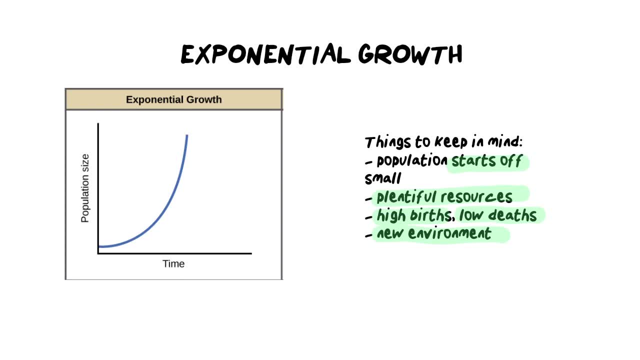 draw it in for you. Essentially, what happens sometimes is a population will dramatically explode, They'll use all their resources and then the numbers just completely go down. They drop off And that might be a breeding cycle. Locusts go through these breeding cycles. 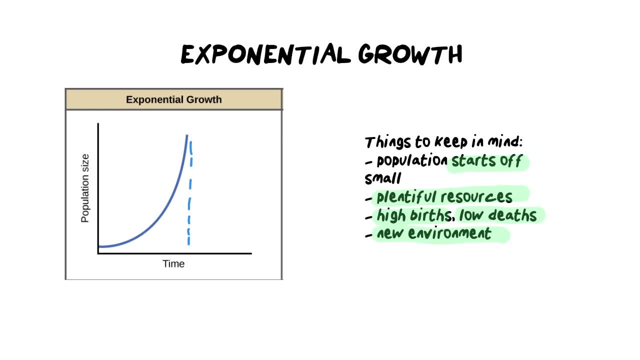 where in the next season that comes around, their population dramatically increases and then they drop off completely. And that is because certain organisms go through these breeding cycles where they've got lots of resources, They use all the resources and then they die, And then they repeat it all over again in the next breeding season. Now we move into 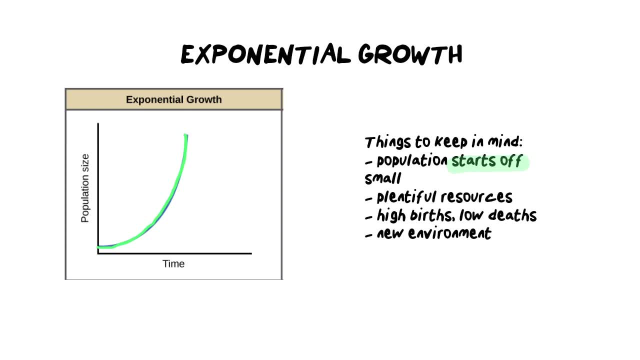 itself is new, and so they are starting off with maybe four or five breeding pairs. There's not going to be a lot of individuals. What's also important in the exponential growth curve is: you must acknowledge that there is plentiful resources. The reason that we know that is because, if we look 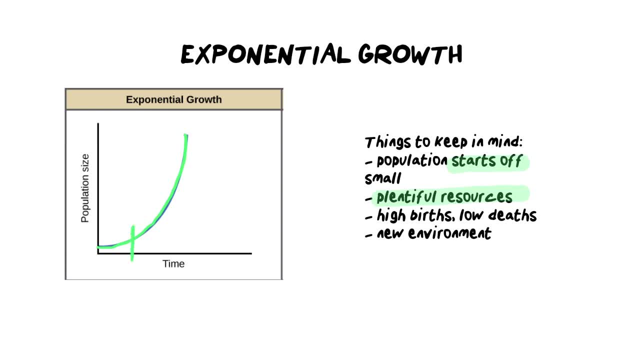 at the graph in the beginning. this figure is going to be the number of individuals that are going to be in the first sector. over here The growth is quite slow and gradual and that is because the amount of breeding pairs are limited and reproduction takes time and you know, just in general populations take 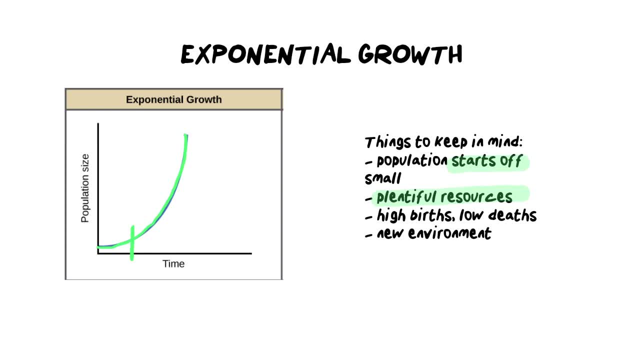 a little while to establish. However, everything after that is exponential, like there's a sharp increase over a very short period of time. That is because there are so many resources available: Very little disease, Very little competition. Everybody has enough of everything to reproduce at their maximum, and so that's why we 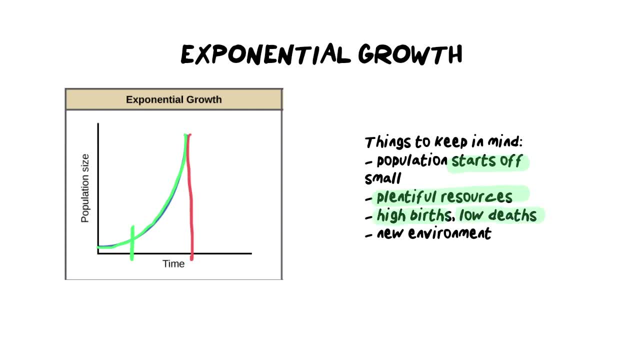 see a high birth, low death rate. Now, the last thing I want you to keep in mind is exponential growth happens often in a new environment. It basically means maybe this organism didn't live there before and now they're newly introduced, or an area that used to have them has been cleared out. 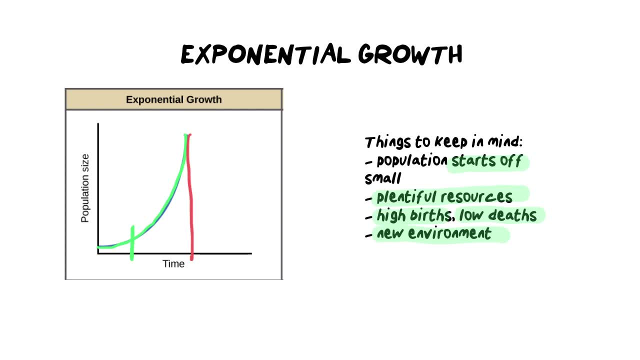 More space has been provided to them and now they have, you know, like an area to establish themselves, And often we see exponential growth in organisms like bacteria. We see these in like rodents and mice or butterflies. There's like an explosion of growth. And then what is missing in? 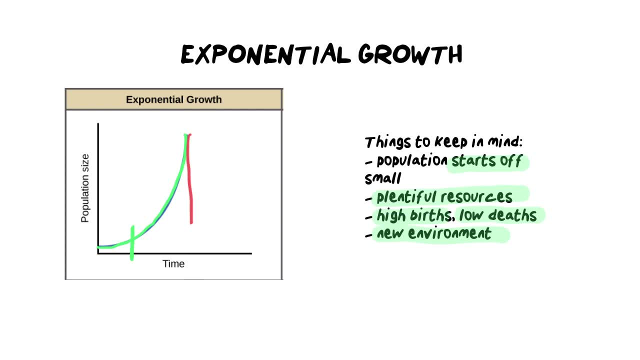 this graph, which I'm going to include for us now, is what we call a drop-off point, And I'm going to draw it in for you. Essentially, what happens sometimes is a population will dramatically explode, They'll use all their resources and then the numbers just complete. 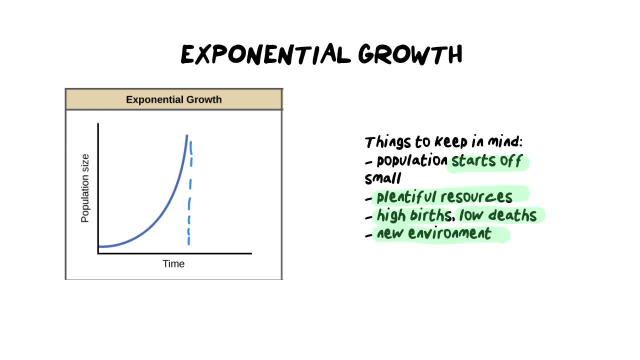 They drop off and that might be a breeding cycle. Locusts go through these breeding cycles where in the next season that comes around, their population dramatically increases and then they drop off completely. And that is because certain organisms go through these breeding cycles. where they've got lots of resources, They use all the resources and then they. 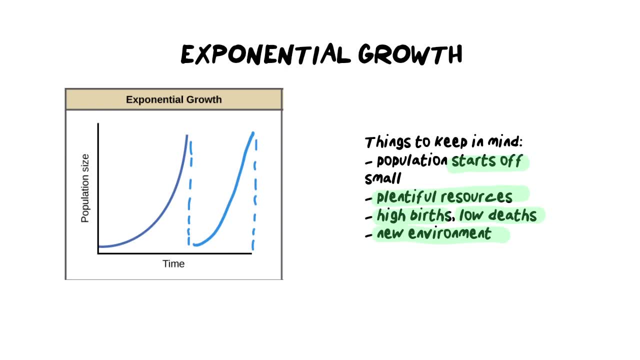 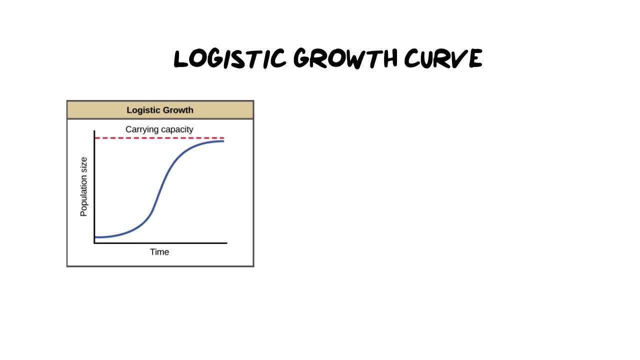 die and then they repeat it all over again in the next breeding season. Now we move into the next growth curve, which follows exponential growth, and that is logistical. Now logistic growth again has a very, very defining shape. You'll notice it has an s shape to it And it's actually 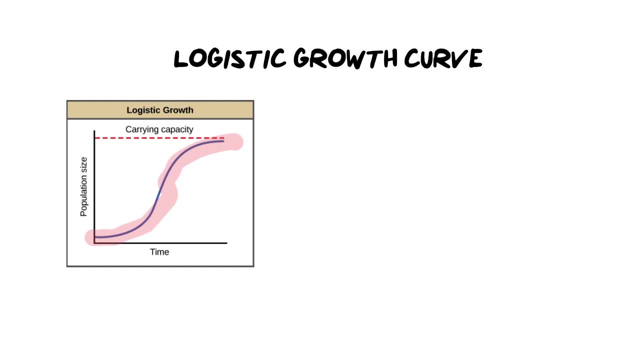 made up of two components, And what I mean by that is it's actually got a couple of phases to it. The first phase we've actually just looked at, which is the exponential growth which happens in the beginning here, But then later on it's followed by the logistical part, which is here. 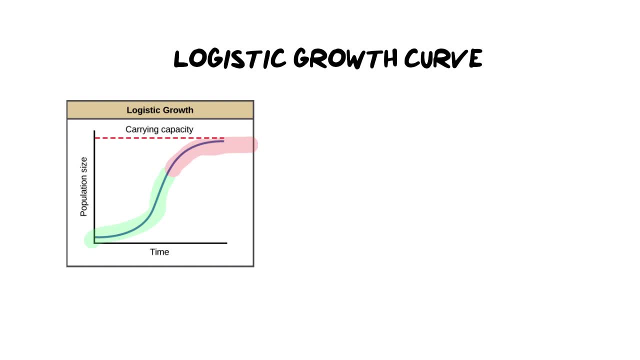 when it starts to level off as well. The second phase is when it starts to flatten. Now again, you are going to need to be able to draw these graphs, label them, and you need to explain what's happening in these populations, And so I'm. 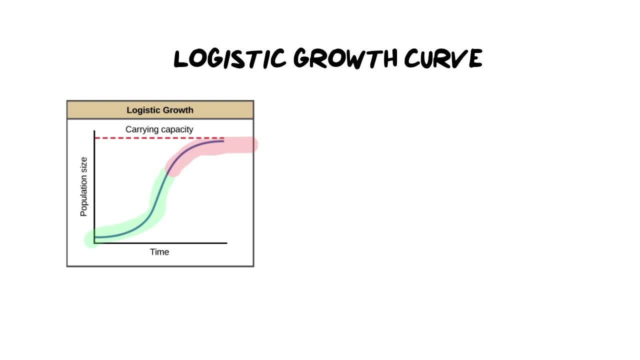 going to give you some things to look out for that you can use to explain yourself in an exam. Now, the most defining feature of a logistical growth curve is, of course, the carrying capacity as we can see it over here, Which we spoke about in the beginning is the maximum amount. 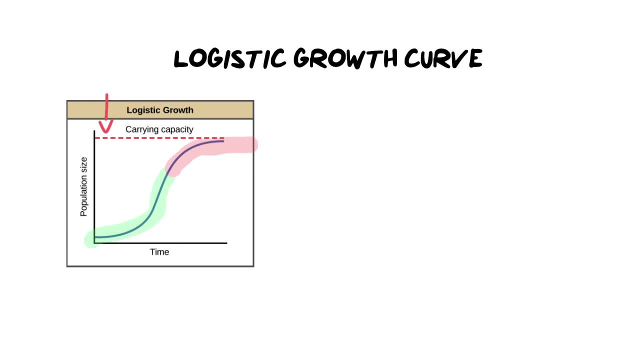 of individuals that we can support And in a logistical growth curve, we have approached the carrying capacity, which means we've gotten up to the maximum number and we've now settled at the maximum number. Sometimes, logistical growth curves can actually do a little bit of a wave all the way along, which is also very 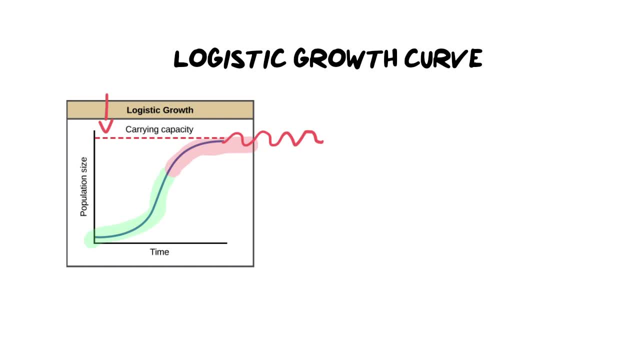 acceptable, because that can happen. So they are not always perfectly flat. at the top is what I'm trying to say and what I would like you to keep in mind. So, when you are explaining logistical growth, these are the things I want you to keep in mind as you explain them. Number one: 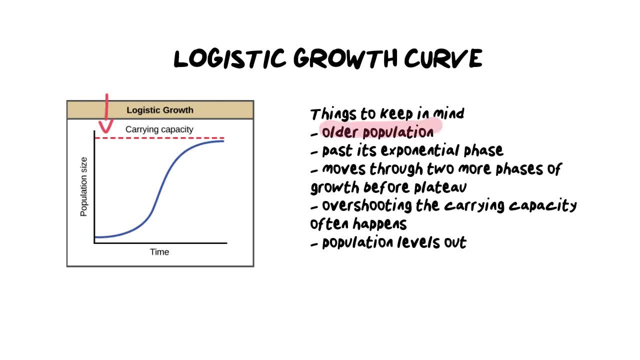 we need to know that this is actually an older population, which means the population has been around for a while, it's established itself, it's gone through already its exponential growth phase. it's now moved into a different phase, a more stable one, And so, because it's past its exponential 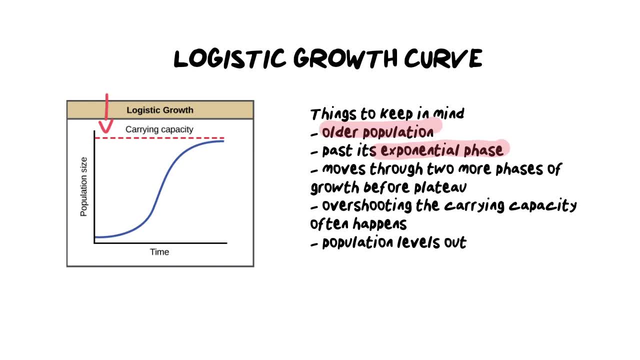 phase. it means that it's not using up all the resources rapidly and it's living very close to the carrying capacity, if not actually on it itself. Now there are two more phases of growth that I want to speak about soon, when we look at the different phases that happen before we get to. 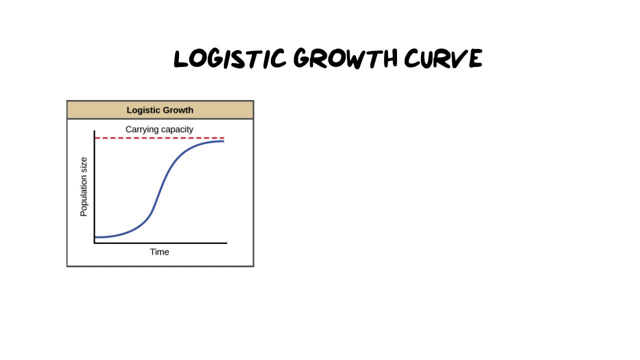 the next growth curve which follows exponential growth, and that is logistical. Now logistic growth again has a very, very defining shape. You'll notice it has an S shape to it And it's actually made up of two components, And what I mean by that is it's actually got a couple of phases to it. 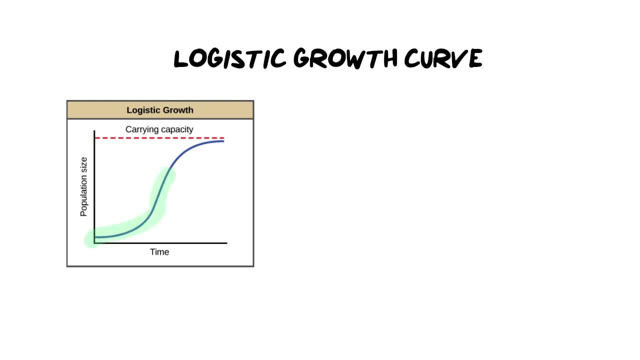 The first phase we've actually just looked at, which is the exponential growth which happens at the beginning here, But then later on it's followed by the logistical part, which is here, when it starts to level off and rise Flatten. Now again, you are going to need to be able to draw these graphs. 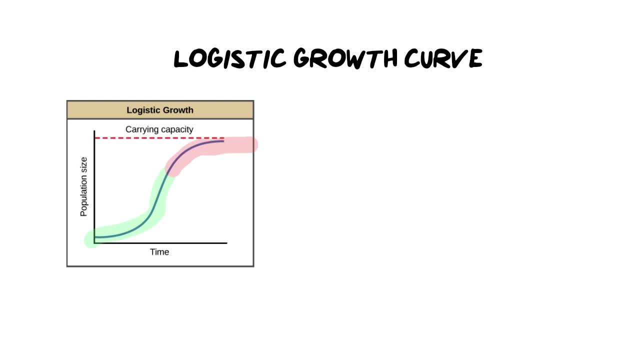 label them, and you need to explain what's happening in these populations, And so I'm going to give you some things to look out for that you can use to explain yourself in an exam. Now, the most defining feature of a logistical growth curve is, of course, the 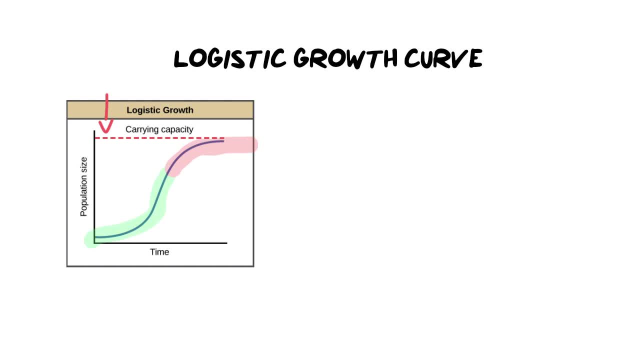 carrying capacity As we can see it over here, which we spoke about in the beginning, is the maximum amount of individuals that we can support And in a logistical growth curve we have approached the carrying capacity, which means we've gotten up to the maximum number and 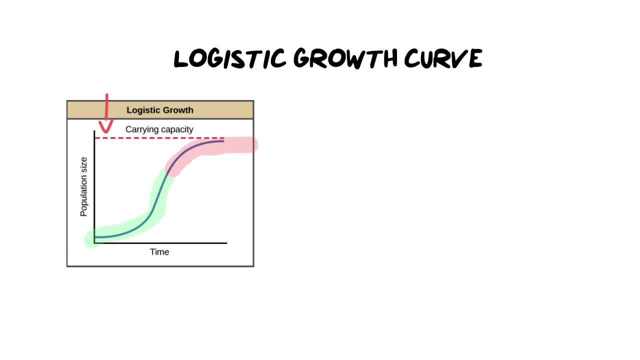 we've now settled at the maximum number. Sometimes logistical growth curves can actually do a little bit of a wave all the way along, which is also very acceptable, because that can happen. So they are not always perfectly flat at the top is what I'm trying to say and what I would like you to keep in. 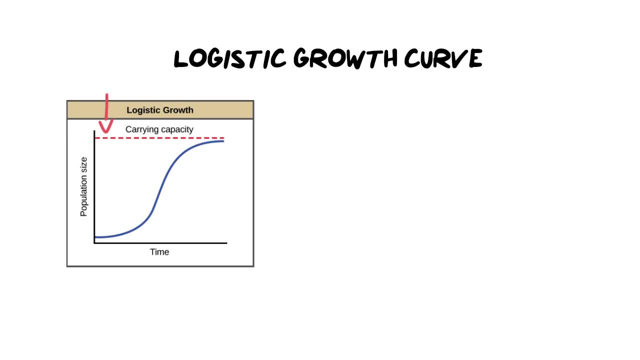 mind. So when you are explaining logistical growth, these are the things I want you to keep in mind as you explain them. First of all, you need to know that this is actually an older population, which means the population has been around for a while, it's established itself, it's gone through already. 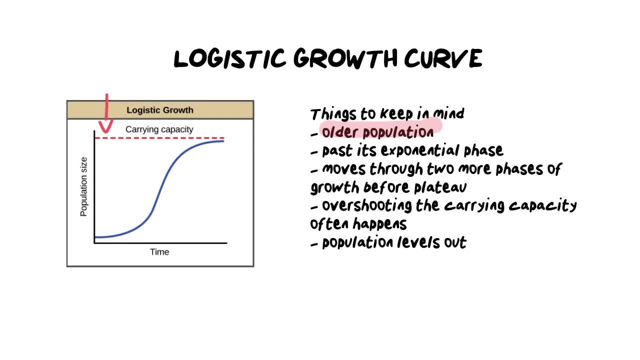 its exponential growth phase, it's now moved into a different phase, a more stable one, And so, because it's past its exponential phase, it means that it's not using up all the resources rapidly, and it's living very close to the carrying capacity, if not actually on it itself. Now there 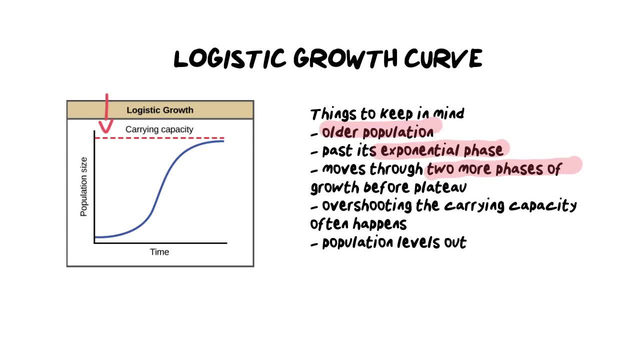 are two more phases of growth that I'm going to show you in a moment. The first one is called the carrying capacity, and it's a phase that I'm going to speak about soon. when we look at the different phases that happen before we get to the plateau- And when I say plateau, 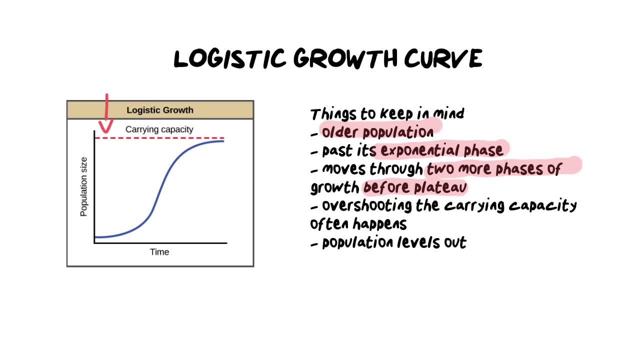 the plateau, And when I say plateau, I'm referring to how the graph can actually start to level out and become flattened like that. Now, that is due to the carrying capacity which, as we mentioned, is created by environmental resistance. Now, sometimes what can happen? as I mentioned to 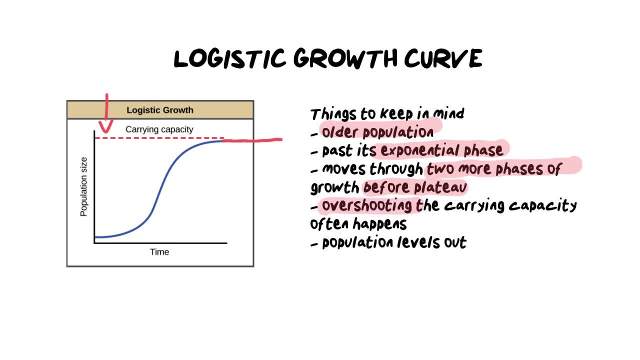 you is, we get what we call an overshooting event, which would look something like this If I were to just take away this line here, and I'm going to continue the graph. what it means is is that sometimes you overshoot the carrying capacity, you drop down past it and then you 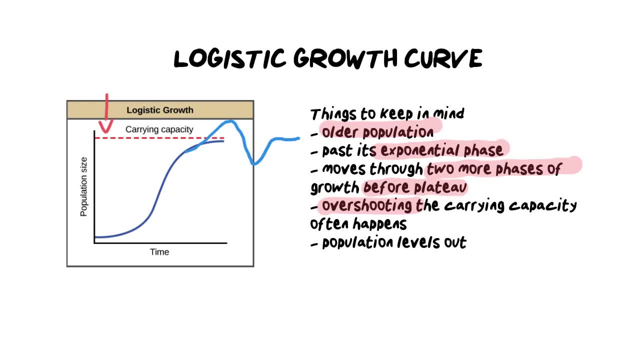 come back up and then you flatten out. This bit over here is called the overshooting event, and essentially it means organisms are rapidly reproducing, making many babies, and then all of a sudden the ecosystem doesn't have any resources to support them. so the ecosystem and 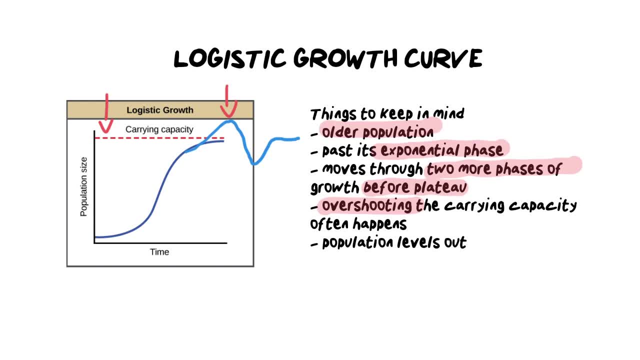 the individuals take a collapse, but the ecosystem recovers and the population can start producing, reproducing again and go back up to where they were before. Now, eventually, the population is going to level out and that is because, remember when you are explaining why does it level out? 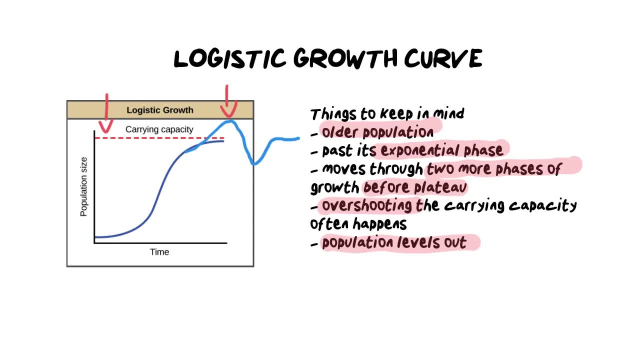 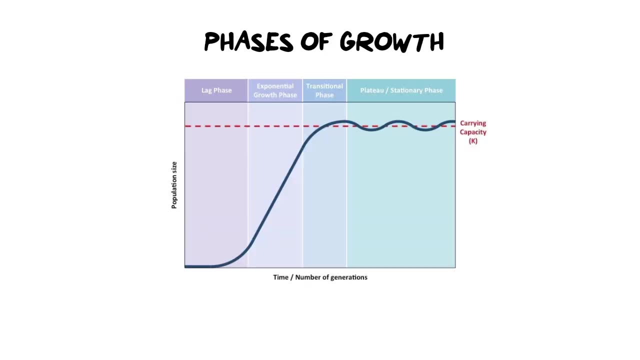 it levels out because environmental resistance has created a carrying capacity which limits the amount of individuals the ecosystem can support and therefore we end up with an end up with a plateau or a stable population curve. Now, as I mentioned to you earlier, you will need to be able to draw these graphs and label them, but not just label them with. 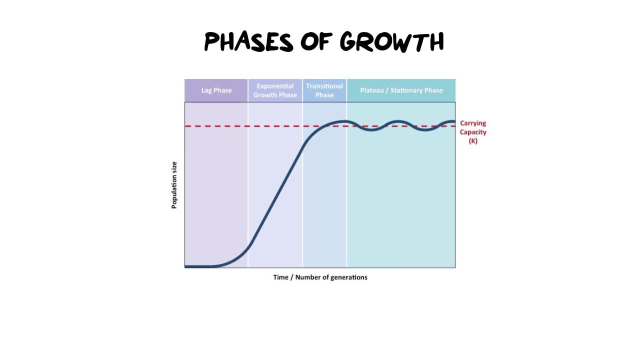 their time and population numbers. you must also be able to identify the phases of growth, in particular logistical growth, because it actually has four phases that you need to be able to identify. So, first of all, we're going to start off with this first phase here, which is the 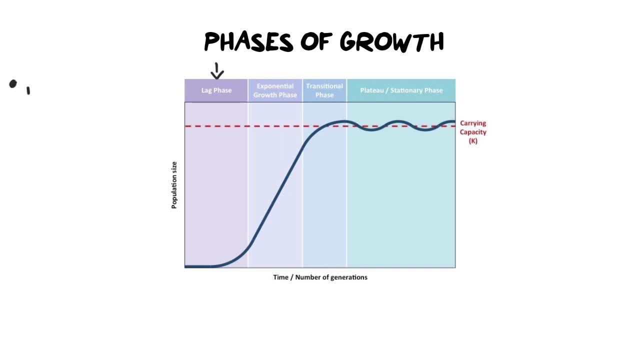 lag phase. Now, the reason why it's called the lag phase is because there are few reproducing couples, and the problem with the lag phase is it takes time to reproduce. it takes time to find a partner to reproduce with. So in the beginning the population growth is very slow and we call it a lag. 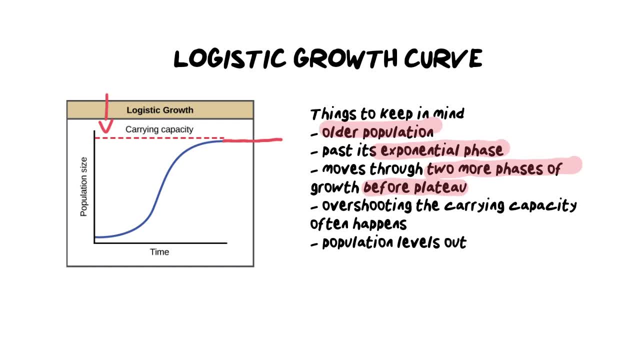 I'm referring to how the graph can actually start to level out and become flattened like that. Now, that is due to the carrying capacity which, as we mentioned, is created by environmental resistance. Now, sometimes what can happen, as I mentioned to you, is we get what we call an overshooting event. 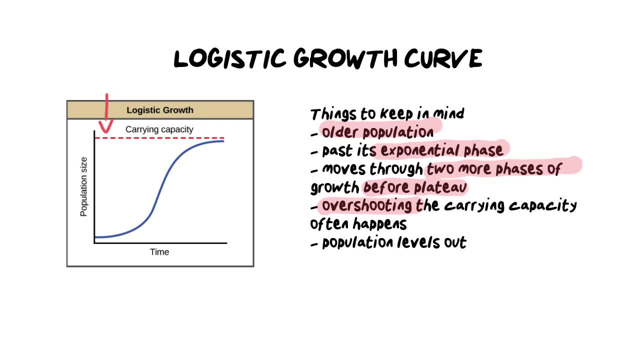 which would look something like this, This line here, and I'm going to continue the graph- What it means is that sometimes you overshoot the carrying capacity, you drop down past it and then you come back up and then you flatten out. This bit over here is called the overshooting event and essentially it means 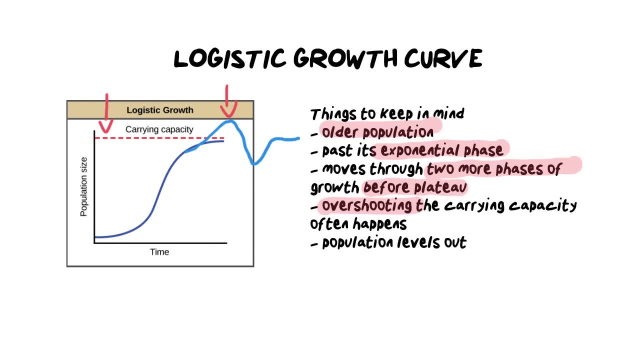 organisms are rapidly reproducing, making many babies, and then all of a sudden the ecosystem doesn't have any resources to support them. so the ecosystem and the individuals take a collapse. But the ecosystem recovers and the population can start producing, reproducing again and go back up. 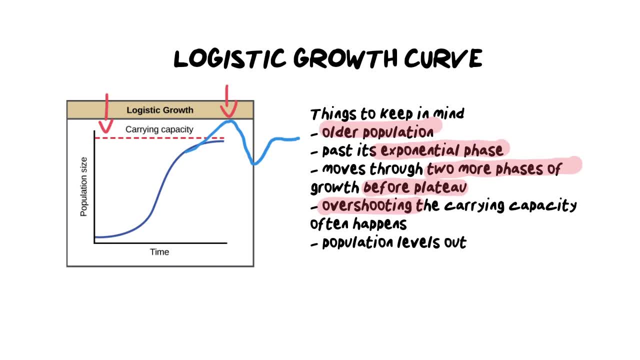 to where they were before. Now, eventually, the population is going to level out and that is because- remember when you are explaining: why does it level out? it levels out because environmental resistance has created a carrying capacity which limits the amount of individuals the ecosystem can support and therefore we end up with a plateau or a state. 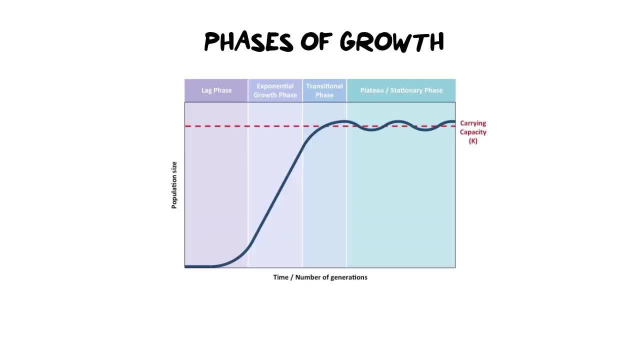 Now, as I mentioned to you earlier, you will need to be able to draw these graphs and label them, but not just label them with their time and population numbers. you must also be able to identify the phases of growth, in particular logistical growth, because it actually has four phases that you need. 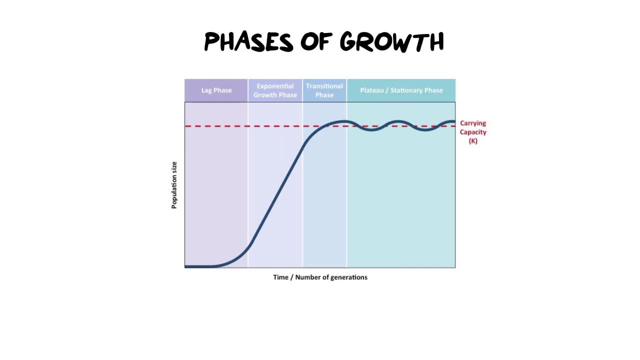 to be able to identify. So, first of all, we're going to start off with this first phase here, which is the lag phase. Now, the reason why it's called the lag phase is because there are few reproducing couples, and the problem with the lag phase is it takes time to reproduce. it takes time to find a partner to. 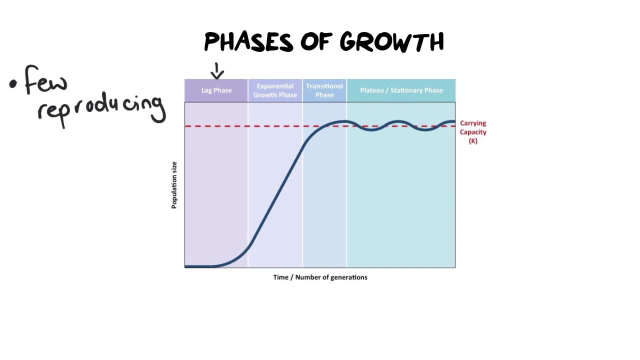 reproduce with. So in the beginning the population growth is very slow and we call it a lag. Then we move into exponential growth. Now, exponential growth means that there are many resources, and of those resources there is also many breeding pairs, and that is why. 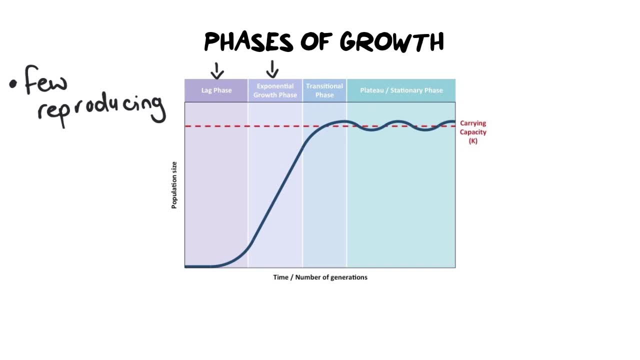 Then we move into exponential growth. Now, exponential growth means that there are many resources, and of those resources there is also many breeding pairs, and that is why you exponentially grow, because at first you were breeding with two individuals. that became four, four, that then became eight, eight, that then became 16.. In the beginning, that's. 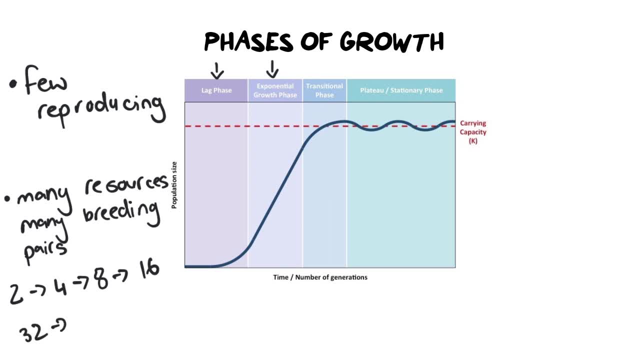 actually quite slow, but after that becomes 32 and then 64 and you see that there's a rapid increase in growth. and that is because you have so many more adults who are mature enough to reproduce and they start replacing themselves exponentially while their own children are still alive. 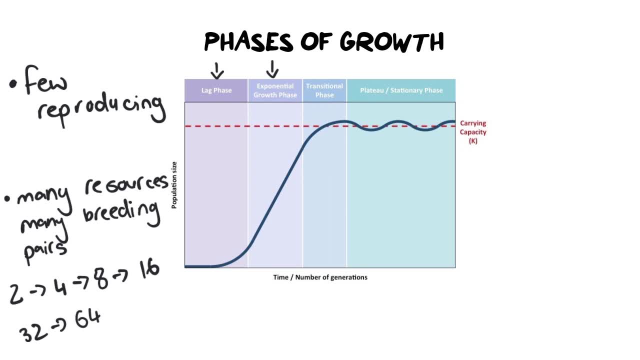 also making babies, and so you have this compacting effect where you add more and more individuals. The next step that we see is the transitional phase, and in your textbook it might be called something different, like the decelerating phase. That's also an acceptable way to describe it as well, but, as the name suggests, this is when 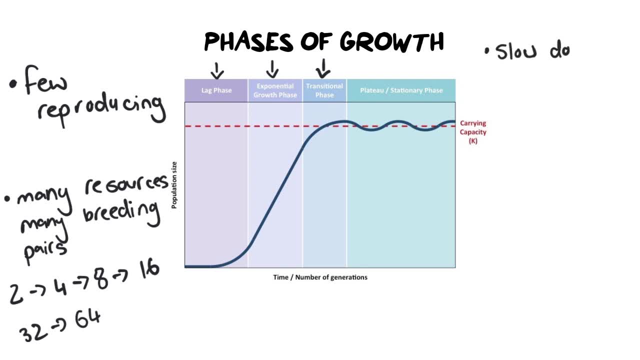 growth starts to slow down, and the reason for that is because, number one, you are approaching the carrying capacity which, if you remember from the beginning of the video, that is the maximum amount of individuals that we can carry, which is shown here by this dotted line, this red dotted. 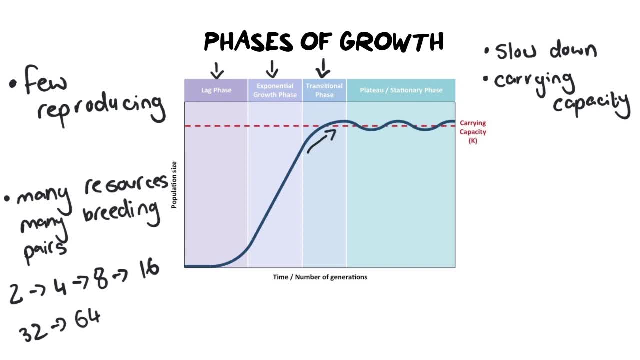 line and as you approach that maximum amount, you are going to slow down in growth because you are running out of resources. so the resources are becoming limited and because they're becoming limited you can have fewer babies, which means that the reproduction rate is slower. you do notice here that the line of the population 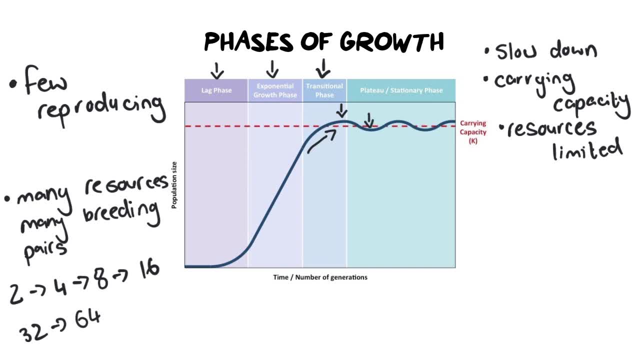 goes just above the carrying capacity and then it dips down below and then it comes back up again and then dips down back a low again, and that's actually quite normal. So you know, some textbooks will have the line go flat, others will have it like fluctuate, like 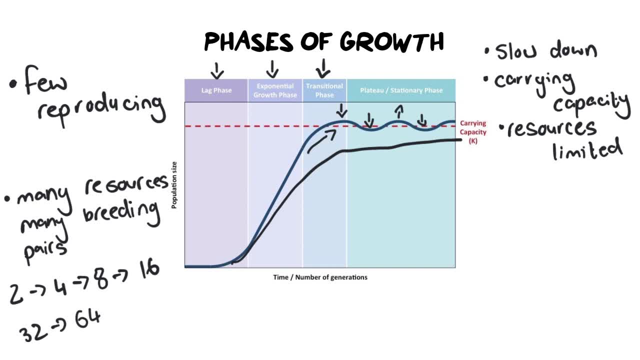 this. they're both correct, but in real life circumstances, most populations do very small fluctuations up and down, which brings me to the final stage, which is what we call the plateau or the stationary phase, and essentially what that is, when we're looking for things, is a population. 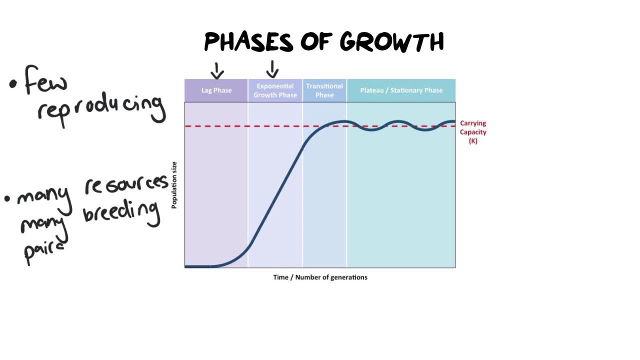 you exponentially grow, because at first you were breeding with two individuals. that became four, four, that then became eight, eight, that then became 16.. In the beginning that's actually quite slow, but after that becomes 32 and then 64 and you see that there's a rapid increase. 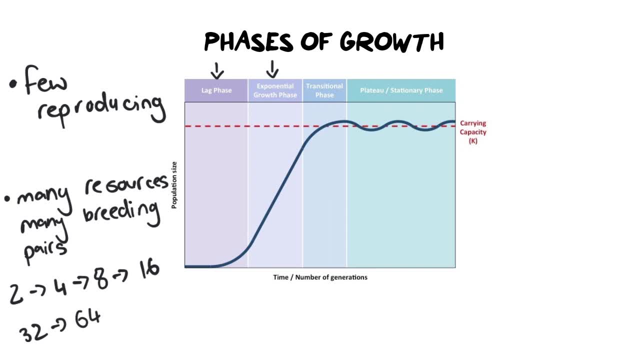 in growth. That is because you have so many more adults who are mature enough to reproduce and they start replacing themselves exponentially while their own children are still alive, also making babies, and so you have this compacting effect where you add more and more individuals. The next step that we see is the transitional phase. 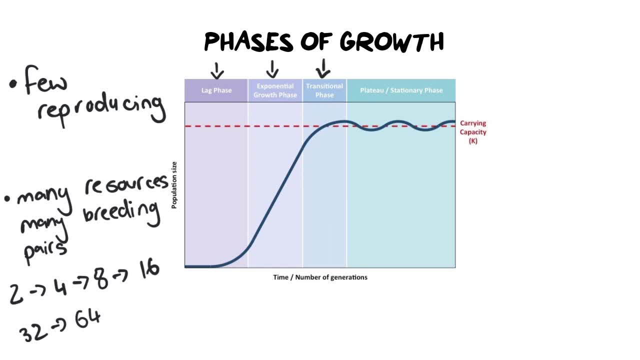 and in your textbook it might be called something different, like the decelerating phase. that's also an acceptable way to describe it as well. But, as the names suggest, this is when growth starts to slow down, and the reason for that is because, number one, you are approaching. 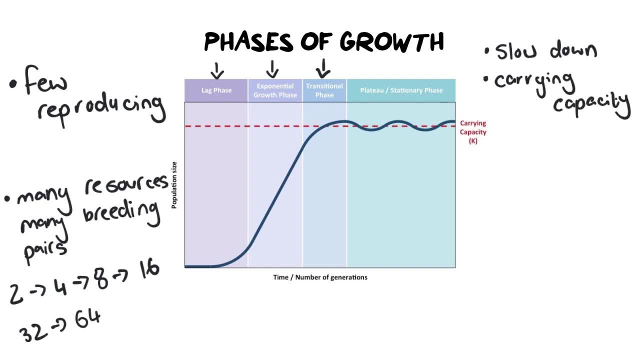 the carrying capacity, That is, the maximum amount of individuals that we can carry, which is shown here by this dotted line, this red dotted line. and as you approach that maximum amount, you are going to slow down down in growth because you are running out of resources. So the resources are becoming 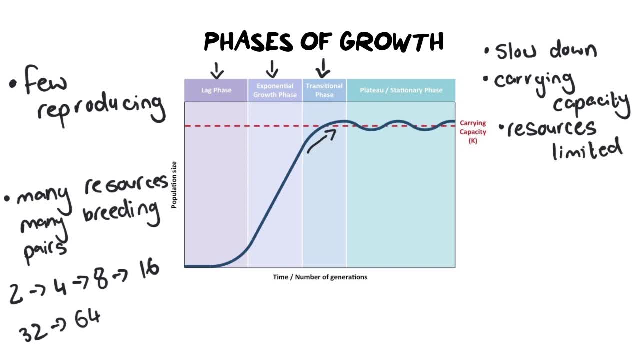 limited, And because they're becoming limited, you can have fewer babies, which means that the reproduction rate is slower. You do notice here that the line of the population goes just above the carrying capacity and then it dips down below, and then it comes back up again and then dips. 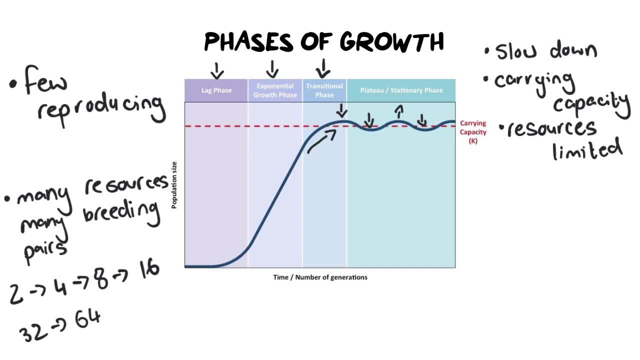 down back below again, And that's actually quite normal. Some tables or some textbooks will have the line go flat, Others will have it fluctuate, like this. They're both correct, But in real life circumstances most populations do very small fluctuations up and down. which brings me to 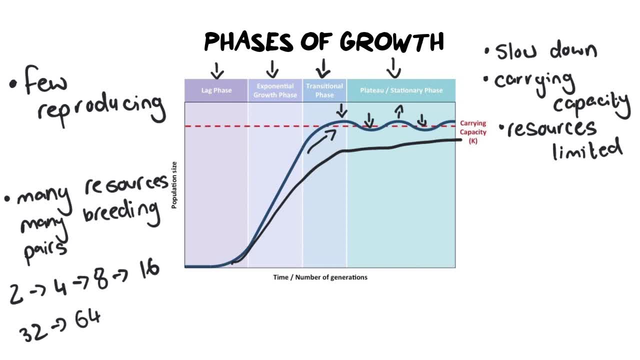 the final stage, which is what we call the plateau or the stationary phase, And essentially what that is, when we're looking for things, is a population that's going to be able to do a lot of things, A population that is fluctuating around the norm, And what that means is you fluctuate. 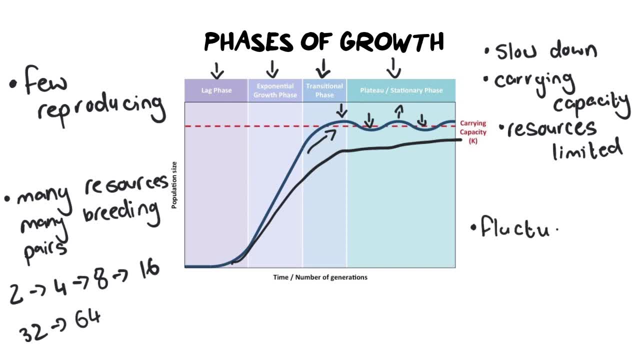 that is fluctuating around the norm, and what that means is you fluctuate around the carrying capacity. and the reason why we become stable is because stability is a result of resources. you have just the right amount of resources to support just the right amount of organism, and so they balance out the 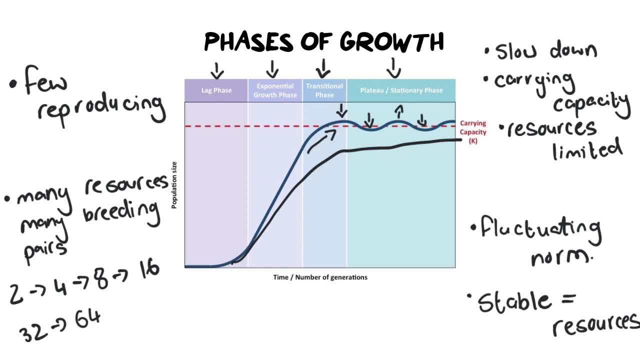 structure of the body With one another. the living components now balance with the non-living components, and that's the maximum amount of individuals an ecosystem can support in a healthy way. I want to remind you, though, that this carrying capacity can, of course, move down if we we lose habitat. it can also move. 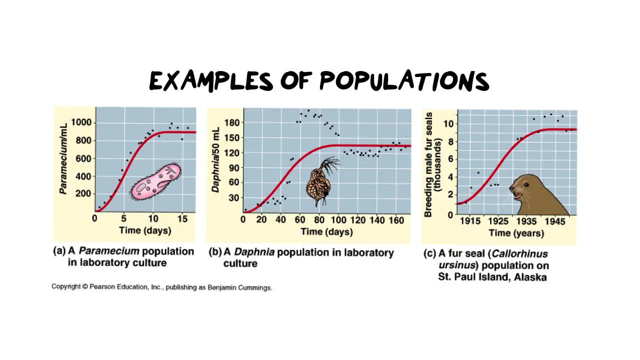 up if we gain habitat. now I just wanted to include some examples of different organisms showing their different populations. all three of these graphs are different species of organisms and I know that because of our S shape that is forming, it shapes slightly different in each of them and I wanted to 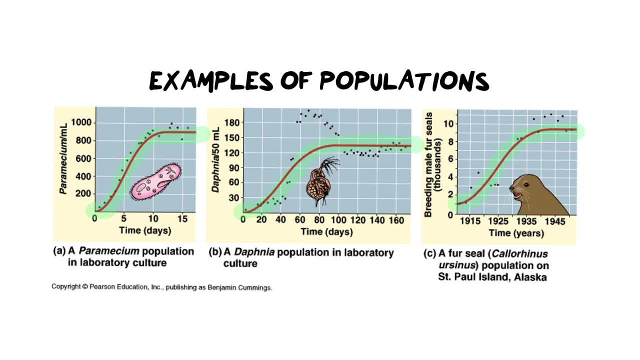 quickly talk about why that is, but essentially they make the same shape. what we have here is a collection of different kinds of organisms. we have a paramecium, we have a Daphina and we have a fur seal. now I wanted to show you the differences between them. 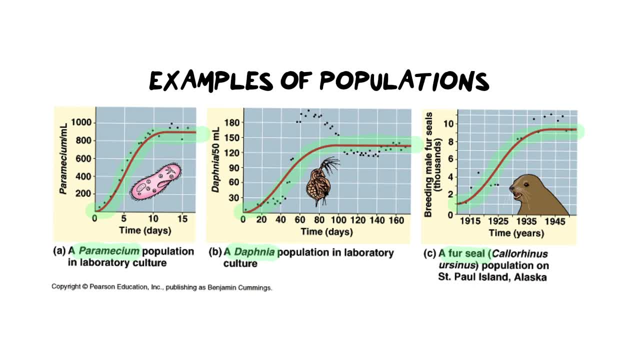 because it's quite interesting, the emphasis or the difference in each of these organisms has to do with how long they live for, and you will notice that for the first two examples, their life cycle and their population cycle is in days, whereas our fur seal here is in years. 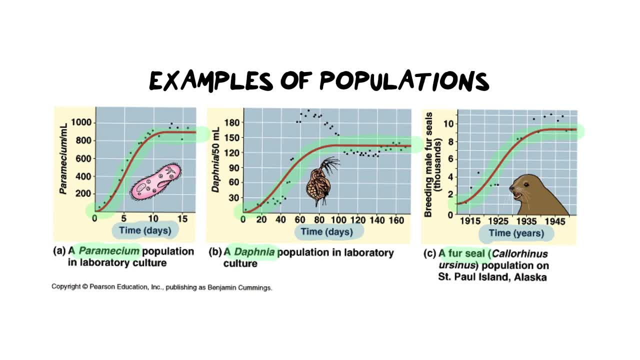 and that's interesting, because what it means is different organisms have different rates of growth when you are unicellular, like our first two organisms here, the paramecium and the Daphenia, they are unicellular, which means that they can grow very, very quickly. another important thing to keep in mind here is: these are both. 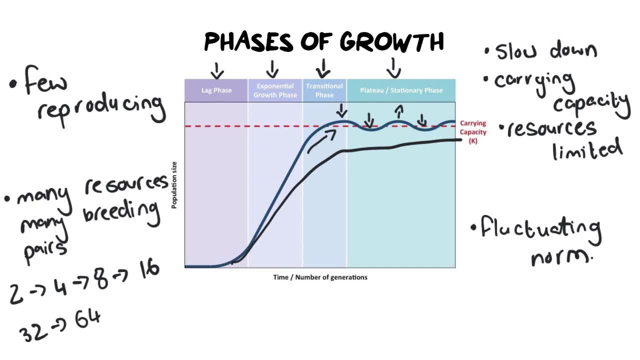 around the carrying capacity, And the reason why we become stable is because stability is a result of resources. You have just the right amount of resources to support your baby, And so you have a population that's going to be able to do a lot of things. 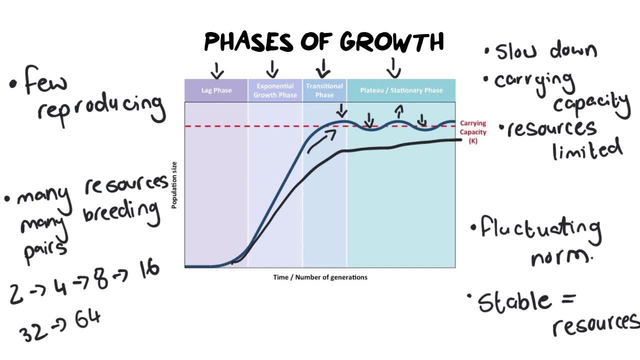 just the right amount of organism, and so they balance out with one another. The living components now balance with the non-living components, and that's the maximum amount of individuals an ecosystem can support in a healthy way. I want to remind you, though, that this carrying capacity 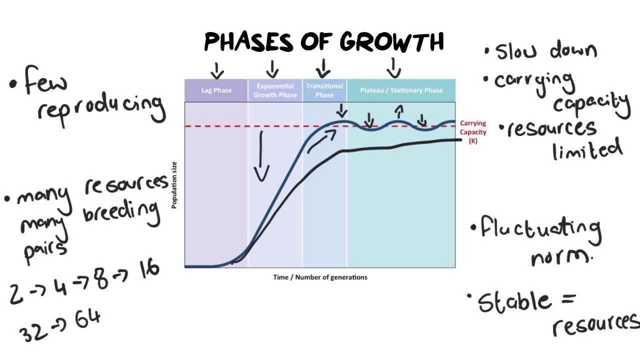 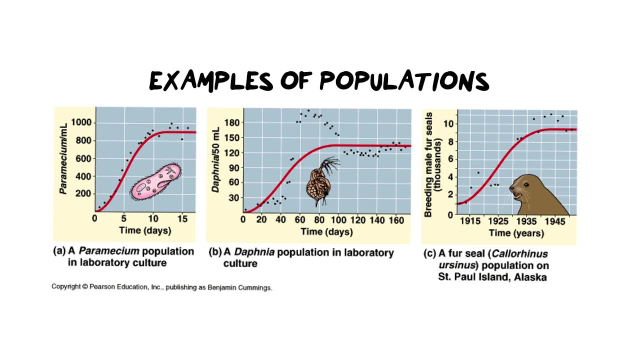 can, of course, move down if we lose habitat. It can also move up if we gain habitat. Now I just wanted to include some examples of different organisms showing their different populations. All three of these graphs are logistical growth, and I know that because of 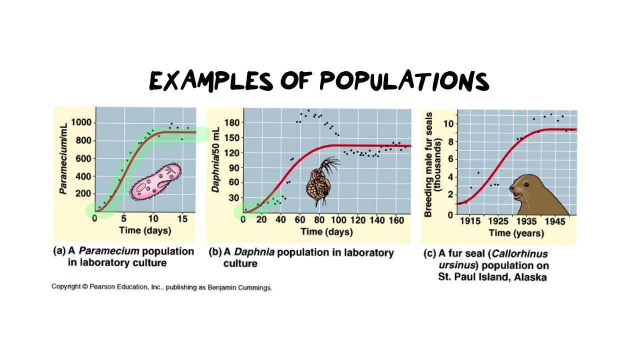 our S shape, that is forming. It shapes slightly different in each of them, and I wanted to quickly talk about why that is, but essentially they make the same shape. What we have here is a collection of different kinds of organisms. We have a paramecium, we have a daphina and we have a 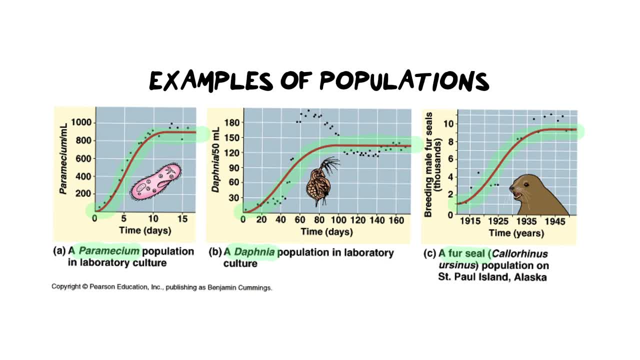 first-stage organism. We have a first-stage organism and we have a first-stage organism. Now I wanted to show you the differences between them because it's quite interesting. The emphasis or the difference in each of these organisms has to do with how long they live for. 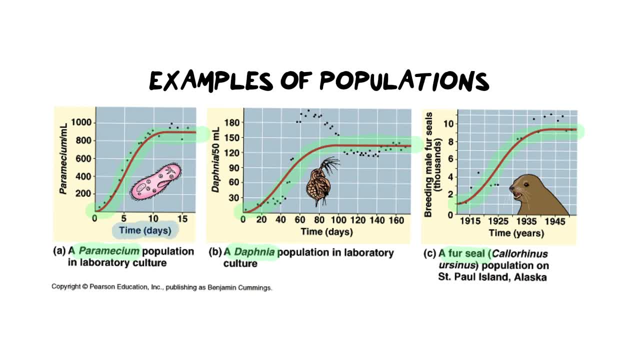 and you will notice that for the first two examples, their life cycle and their population cycle is in days, whereas our first seal here is in years. and that's interesting because what it means is different organisms have different rates of growth When you are unicellular. 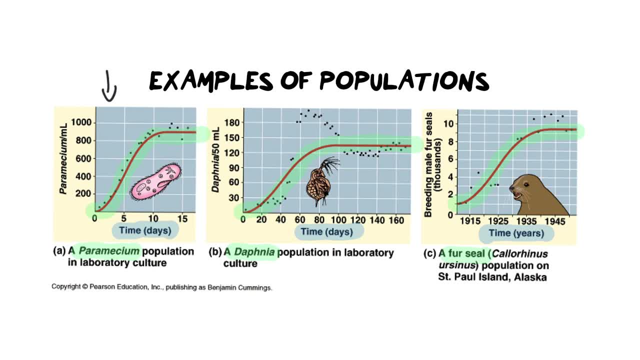 like our first two organisms here, the paramecium and the daphina, they are unicellular, which means that they can grow very, very quickly. Another important thing to keep in mind here is these are both laboratory examples, which means they are placed in prime conditions, and that means 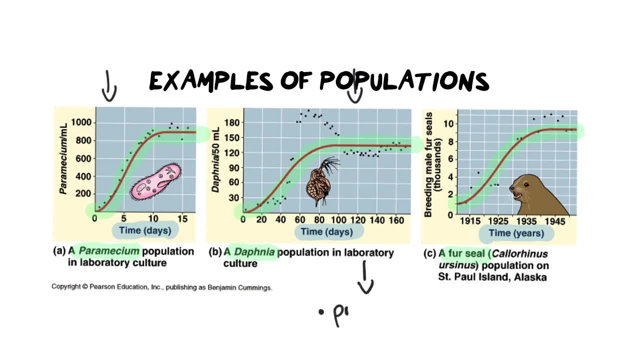 laboratory examples, which means they are placed in prime conditions and that means they have lots of food, lots of space. they don't have any diseases or anyone else to compete with. you know no other species to compete with, so that's also something to keep in mind- versus our little fur seal here which is out in the wild and in nature. 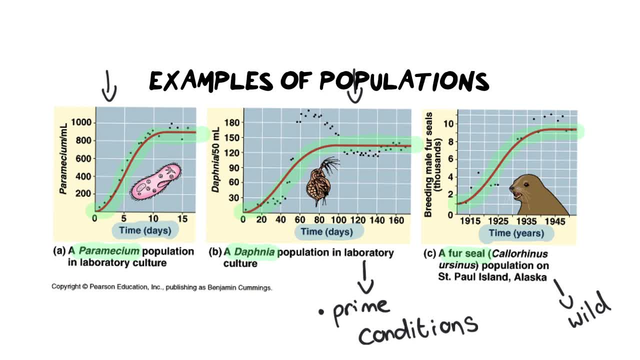 that was what we came up with. this is where we started to use this word fur seal, and when we made this next slide. there are a lot of examples of what we found in the past, what you need to keep in mind when you discuss these kinds of things and you discuss the steepness. 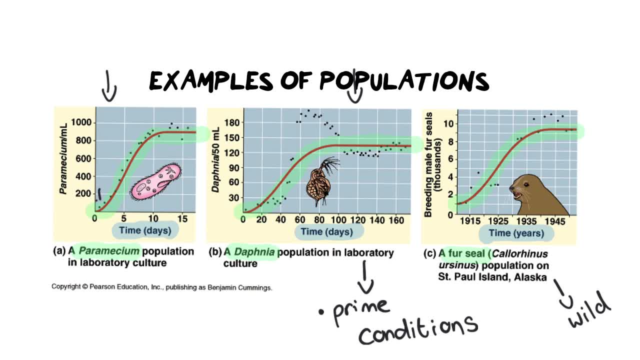 of the graph, You will notice. they all have a lag period, which is when each of these populations is establishing themselves. They all have an exponential growth point, some steeper than others, and that means technically the paramecium is very steep, because this is over five and ten. 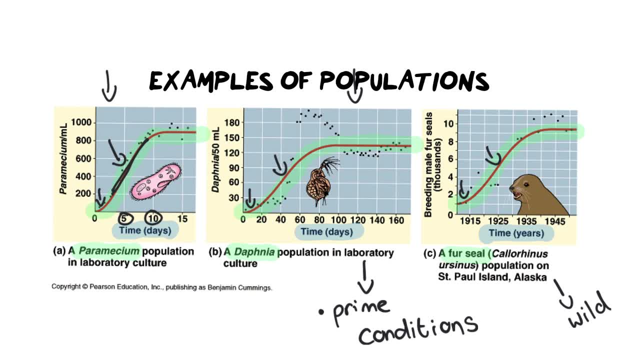 days they have their greatest increase. If you compare it to our seals, they actually have their most exponential growth over here and that is about from, let's say, 1920 to 19,. let's say 30. So over a 10-year period they have had their exponential growth versus five days. So it's 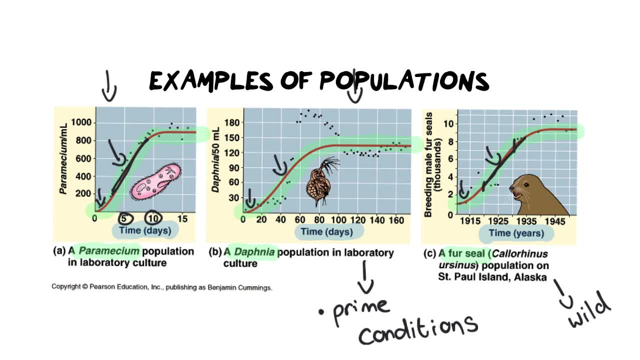 really important that you are able to read the graph properly when you're explaining how they have their greatest increase. So if you compare it to our seals, they actually have different types of animals grow. They also all have a decelerating point, As you can see here. 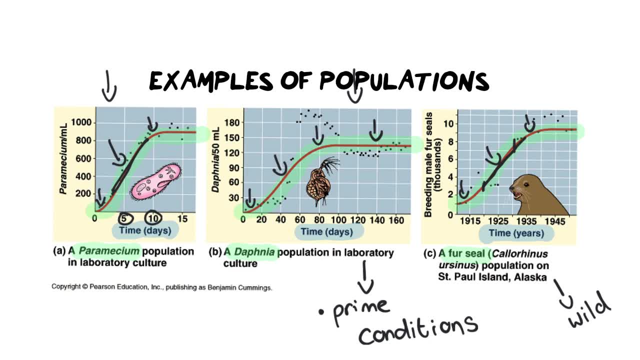 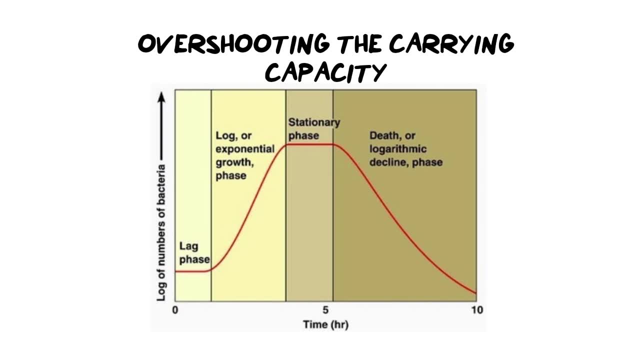 they're slowing down, and then they all have a plateau or a point that they level off on. Now, the final thing I want to discuss is what happens if you overshoot the carrying capacity but you don't recover, And so we, at this point, have only discussed the following, which is a 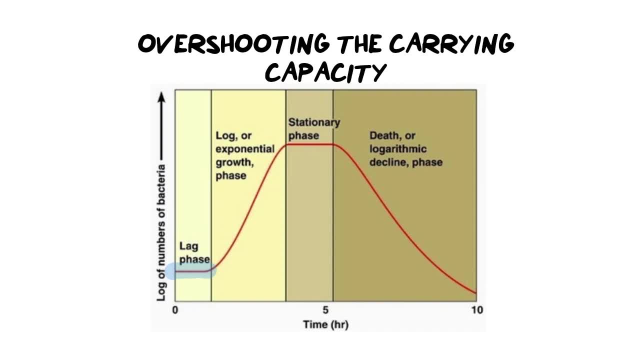 population establishes itself in the lag phase or the establishing phase. It exponentially grows, it slows down and it becomes stationary. For now, that's what we have discussed. And when it becomes stationary like that, we need to remember that there is a portion of the carrying capacity. 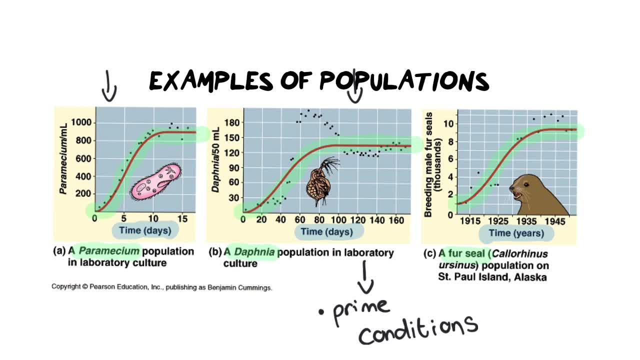 they have lots of food, lots of space. They don't have any diseases or anyone else to compete with other species to compete. So that's also something to keep in mind- versus our little first seal here, which is out in the wild and in nature. That was what you need to keep in mind when you discuss these kinds of things. 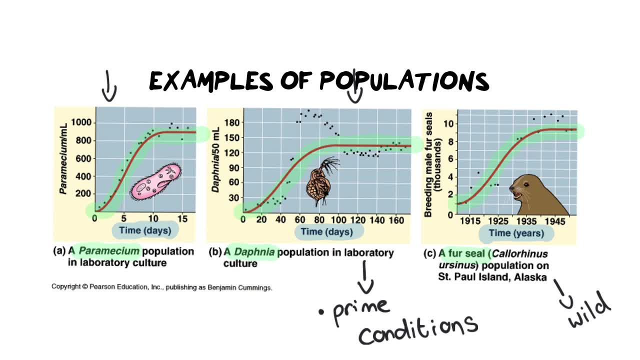 and you discuss the steepness of the graph, You will notice they all have a lag period, which is when each of these populations is establishing themselves. They all have an exponential growth point, some steeper than others, and that means technically the paramecium is very steep because this is over five and ten days. they have their greatest. 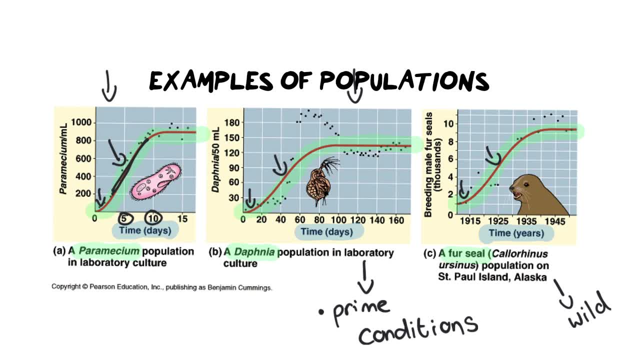 increase. If you compare it to our seals, they actually have their most exponential growth over here and that is about from, let's say, 1920 to 1930.. So over a 10-year period they have had their exponential growth versus five days. So it's really important to keep in mind that these are. 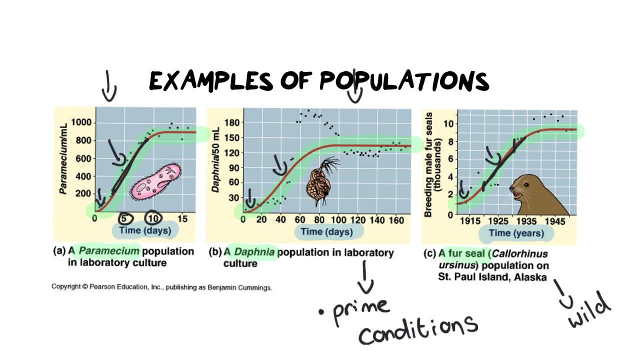 different types of animals and it's important that you are able to read the graph properly when you're explaining how different types of animals grow. They also all have a decelerating point, As you can see here. they're slowing down and then they all have a plateau or a point that they 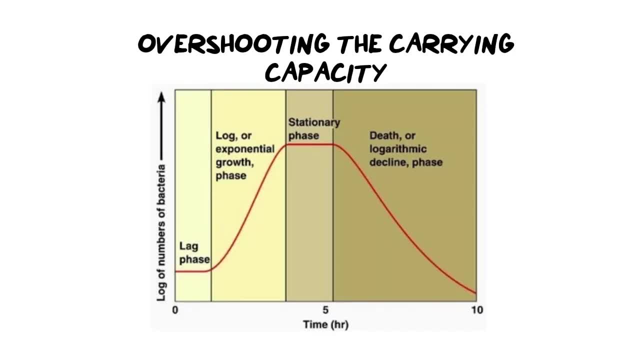 level off on Now. the final thing I want to discuss is what happens if you overshoot the carrying capacity but you don't recover, And so we, at this point, have only discussed the following, which is a population establishes itself in the lag phase or the establishing phase. 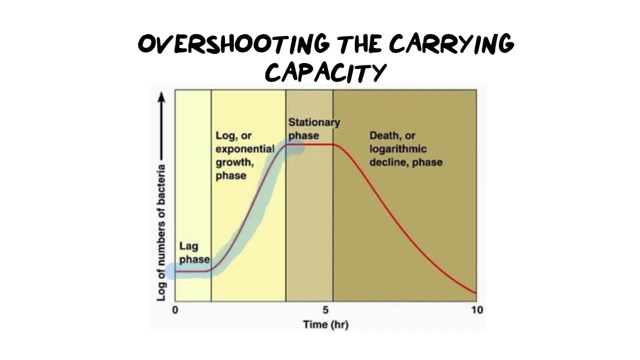 It exponentially grows, it slows down and it becomes stationary. For now that's what we have discussed, And when it becomes stationary like that, we need to remember that there is a portion of the carrying capacity that we can't see here, which I'm just going to put here in a dotted line. 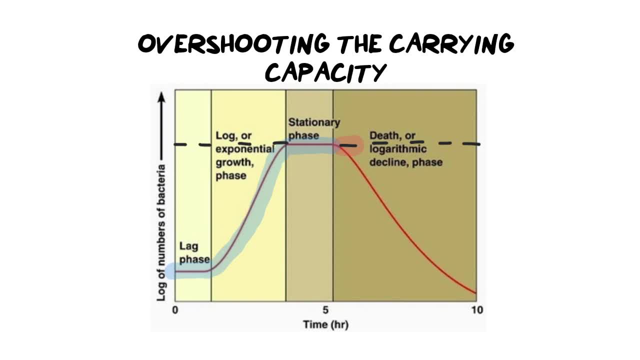 that we can't see here, which I'm just going to put here in a dotted line. That is where that is. In this newer graph, though, I have added in the death or the decline phase that you can see here, And essentially that is illustrating. 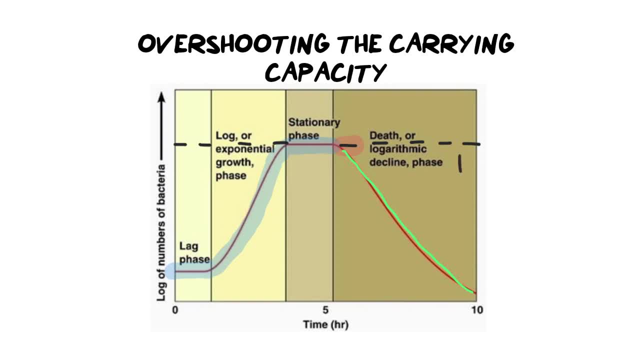 what happens if the carrying capacity continues to drop and does not return back up to where it was before? In other words, there has been some major event. Now this major event could be independent or dependent on the density. So what that means is: maybe we have used up all the resources, so all the food is gone. 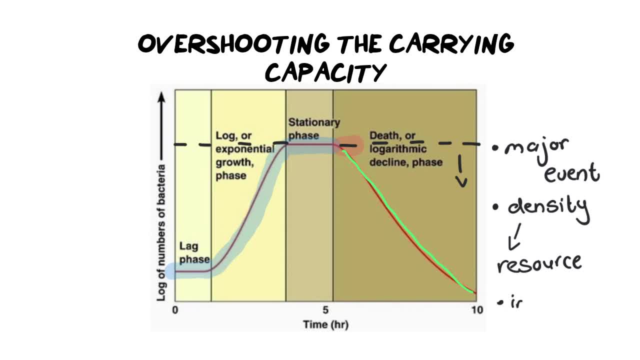 or it might be independent, which means it has nothing to do with how big the population is, And that could be something like a natural disaster, maybe like a flood or a fire, And what can happen is an entire ecosystem can disappear, The carrying capacity lowers and gets lower and lower, And so what we're going to do is we're going to do a little bit of a fossilization, So we're going to get rid of the food and we're going to get rid of the food, and we're going to get rid of the food And then we're going to get rid of the food. So it's. 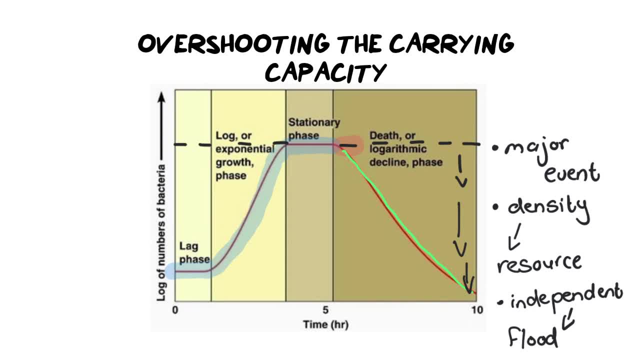 going to get lower and lower and lower, because it cannot support the organisms and they end off dying and becoming extinct. So this would be at the bottom here, an extinction point. This organism has become extinct In this particular graph. this is a bacterial population, So don't. 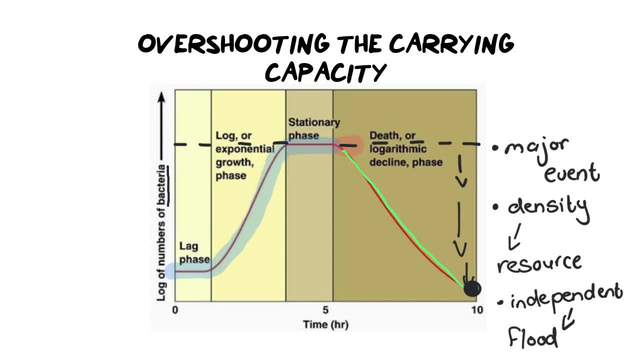 forget to make sure you familiarize yourself with what organism this is. This is bacteria And this is what we see in hours, So this is about a 10-hour period And this is very, very, very possible. and in my experience of how I'd explain this is, this is probably a resource issue. If we were 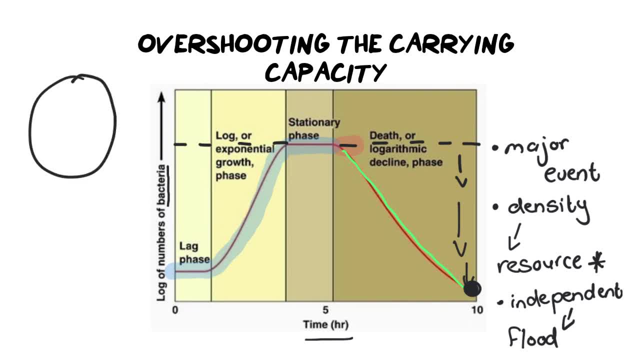 growing bacteria in a petri dish. they have a limited amount of space right, Which means they also have a limited amount of resources. So once the bacterial population starts to grow- and let's imagine each of these dots is the bacteria growing and reproducing Once they take up all the space. 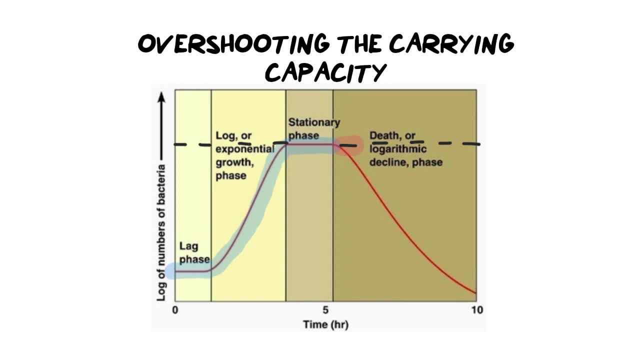 That is where that is. In this newer graph, though, I have added in the death or the decline phase that you can see here, And essentially that is illustrating what happens if the carrying capacity continues to drop and does not return back up to where it was before. In other words, there has been some major event. 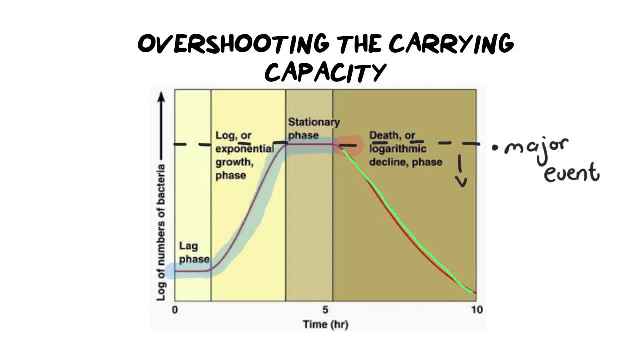 Now, this major event could be independent Or dependent on the density. So what that means is maybe we have used up all the resources, So all the food is gone, Or it might be independent, which means it has nothing to do with. 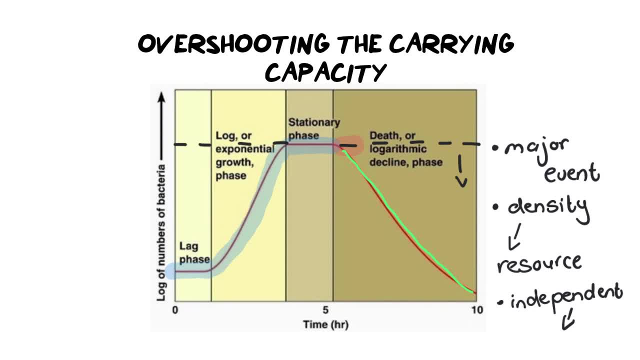 how big the population is, And that could be something like a natural disaster, maybe like a flood or a fire, And what can happen is an entire ecosystem can disappear. The carrying capacity lowers and gets lower and lower and lower because it cannot support the organisms. 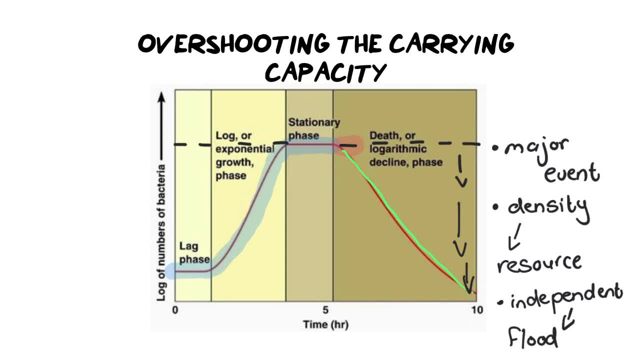 And they end off dying and becoming extinct. So this would be at the bottom here, an extinction point. This organism has become extinct In this particular graph. this is a bacterial population, So don't forget to make sure you familiarize yourself with what organism this is. This is bacteria. 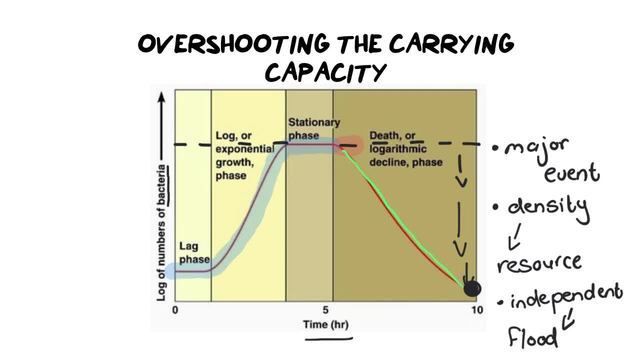 And this is what we see in hours. So this is about a ten-hour span, So you won't have to get to you know 10 days if you left, And I think that is a long term perspective on how we are going to see what happens. So this is just information. 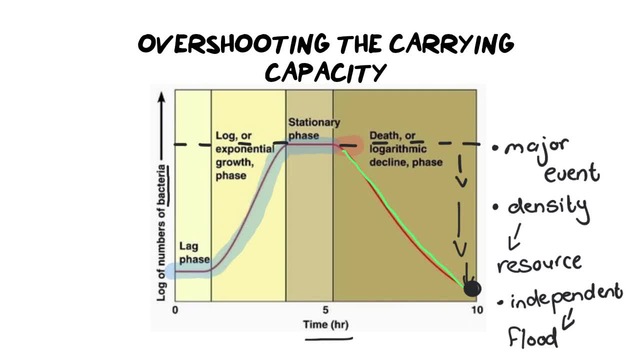 And then after the longer period, that is in some ways, what we are going to see and how things are going to happen, But at the end of the day, there is aшей hour period And this is very, very, very possible. And in my experience of how I'd explain this is: 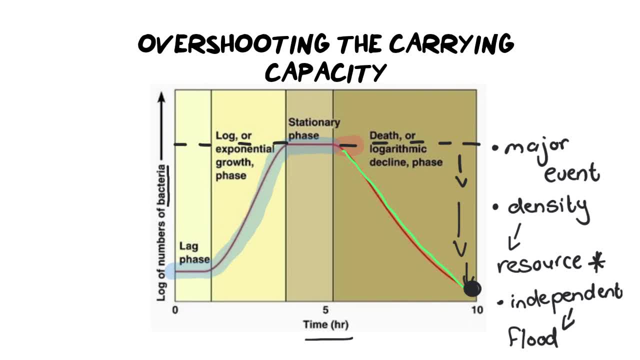 this is probably a resource issue. If we were growing bacteria in a Petri dish, they have a limited amount of space right, Which means they also have a limited amount of resources. So once the bacterial population starts to grow- and let's imagine, each of these dots is the 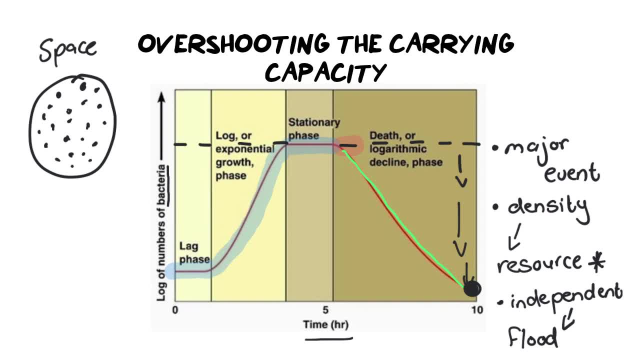 bacteria growing and reproducing. Once they take up the all the space and all the resources in the dish, what you will find is a mass sort of death event where all of these bacteria start to die And there's no way for new resources to be added in a Petri dish right, Because a Petri dish is. 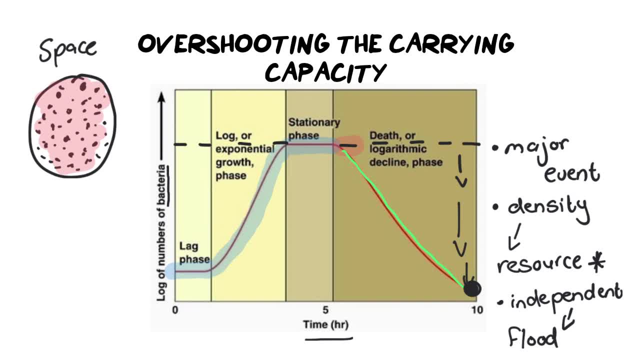 fixed. It's not alive, it's not growing, it is a isolated space, And so that is how you can overshoot carrying capacity in the lab. you can also do it in real life, as I mentioned to you, you might. 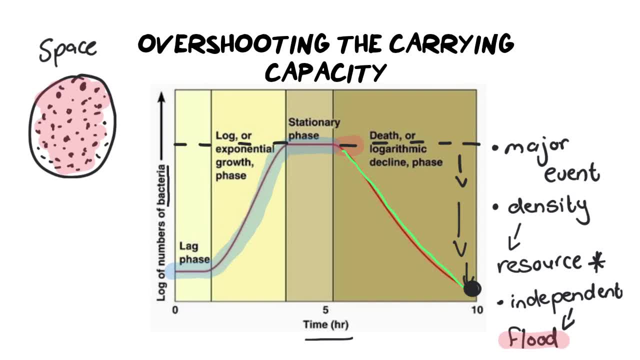 have some kind of flood or fire, Or you could have global warming, which is a slightly longer process but still results in extinction, Or, ultimately, you could have a disease that kills all the females. you're only left with males, And that means that males can't reproduce without. 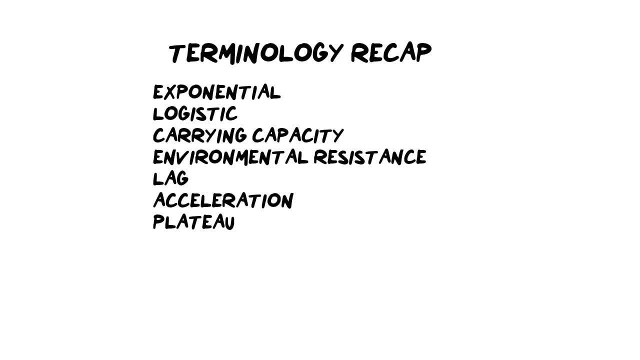 females, So the population becomes extinct. Now, as always, I like to finish off my section with a question, A terminology recap. please use these words to study from for flashcards, But also these are the words that you should be using when you are describing growth in graphs. First of all, we get 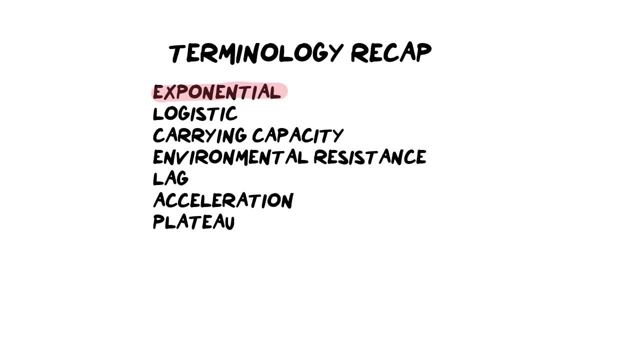 two major kinds of graph. we get the exponential graph, which is the graph where we see slow growth followed by a rapid burst of growth, and it is continuing to grow. it has not reached its peak yet. That is then followed by the logistical growth curve, which is when exponential growth is. 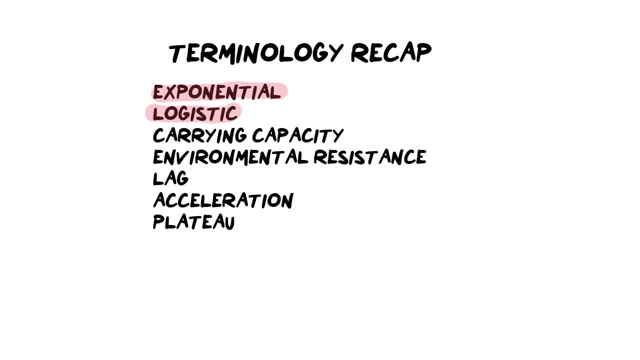 occurring, but now it's being followed by a period of stability and the growth is slowing down and becoming flat like a plateau. Now, what creates that plateau, what creates a logistical graph shape, is the carrying capacity, which is the maximum amount of individuals a ecosystem can. 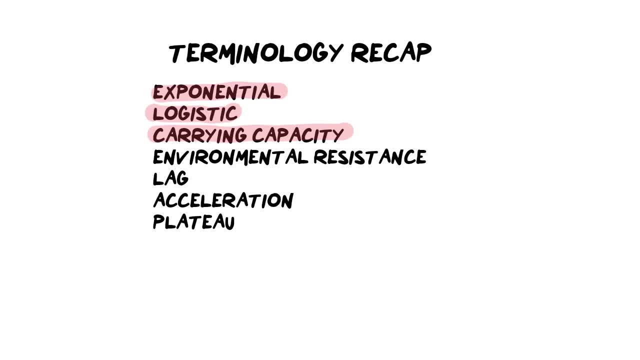 support. So as you move towards the carrying capacity, the graph will become flatter. And who makes this carrying capacity is something known as environmental resistance. So if you have a graph like this, you can see that this graph is called the environmental resistance, which is 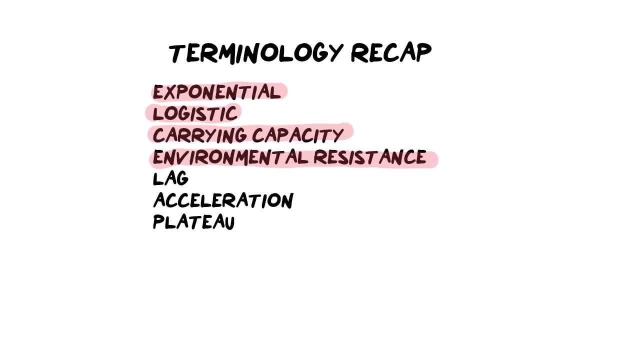 essentially the environment resisting the growth of the population. And the environmental resistance is things like space, water, shelter, mates, soil if you're a plant, and light if you're a plant. these are all the things that, if we calculate them all together, it will give us a number of how many. 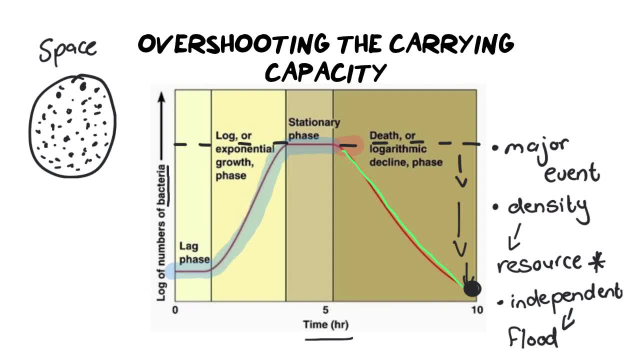 and all the resources in the dish, what you will find is a mass sort of death event where all of these bacteria start to die And there's no way for new resources to be added in a petri dish right, Because a petri dish is fixed, It's not alive, it's not growing, it is a isolated space. 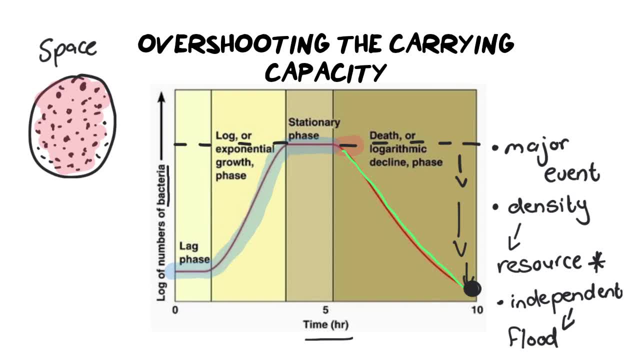 And so that is how you can overshoot the carrying capacity in the lab. You can also do it in real life. As I mentioned to you, you might have some kind of- you know, you might have some kind of flood or fire, or you could have global warming, which is a slightly longer process, but still. 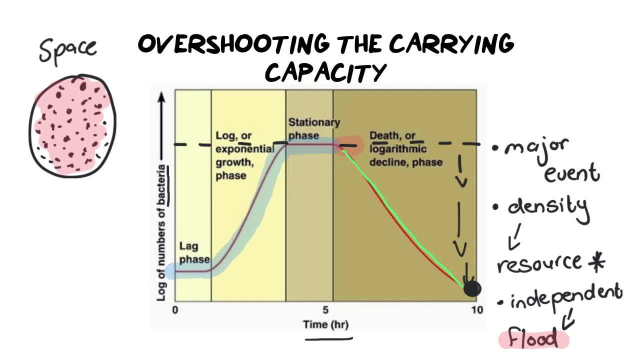 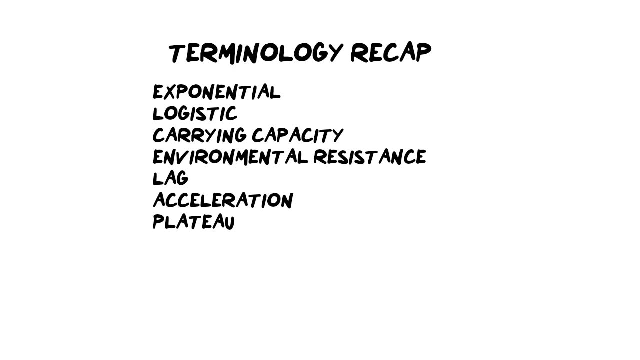 results in extinction, Or ultimately, you could have a disease that kills all the females. you're only left with males, And that means that males can't reproduce without females, So the population becomes extinct. Now, as always, I like to finish off my section with a terminology recap, please. 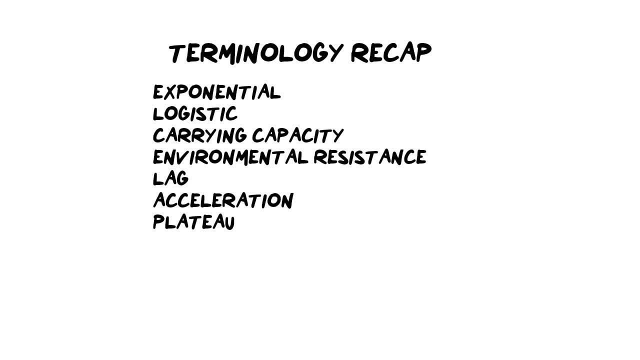 use these words to study from for flashcards, But also these are the words that you can use to, that you should be using when you are describing growth in graphs. First of all, we get two major kinds of graph. we get the exponential graph, which is the graph where we see slow growth. 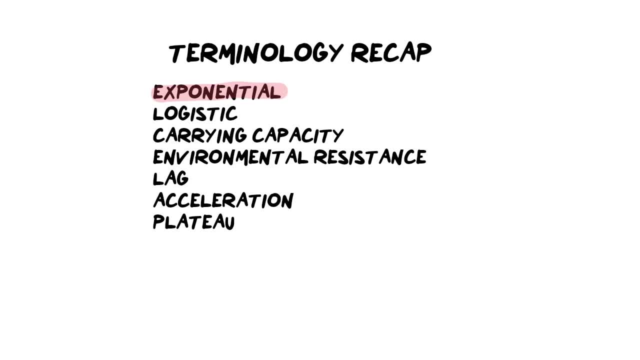 followed by a rapid burst of growth, and it is continuing to grow. it has not reached its peak yet. That is then followed by the logistical growth curve, which is when exponential growth has occurred, but now it's being followed by a period of stability and the growth is slowing. 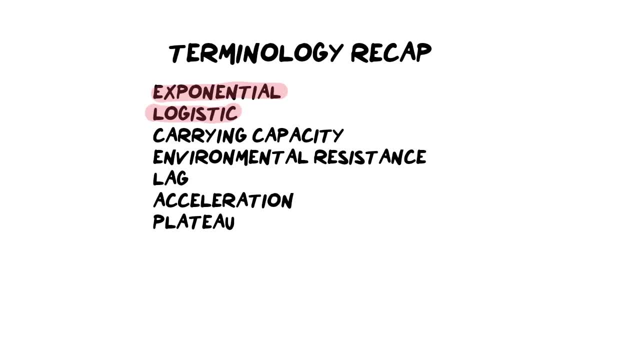 down, And so that's the first thing that we're going to look at, And then we're going to look at and becoming flat like a plateau. Now, what creates that plateau, what creates a logistical graph shape, is the carrying capacity, which is the maximum amount of individuals a ecosystem can. 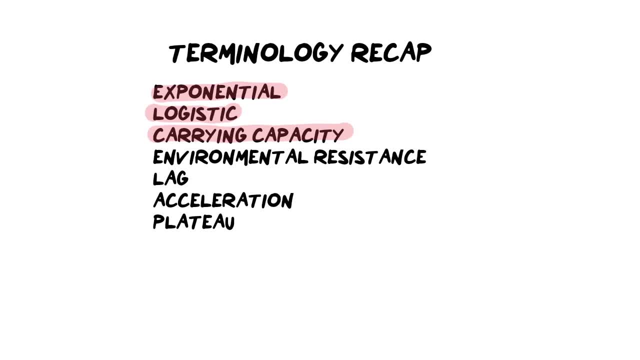 support. So as you move towards the carrying capacity, the graph will become flatter. And who makes this carrying capacity is something known as environmental resistance, which is essentially the environment resisting the growth of the population, And the environmental resistance is things like space, water, shelter, mates, soil. if you're a